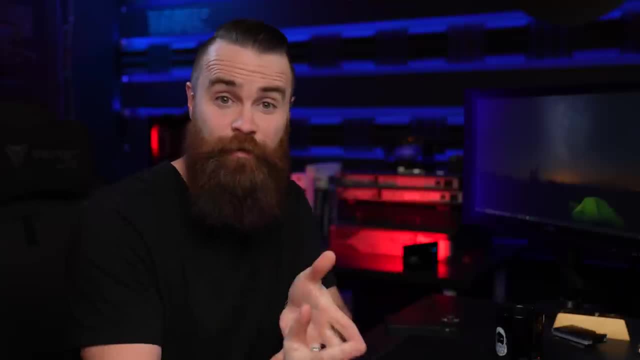 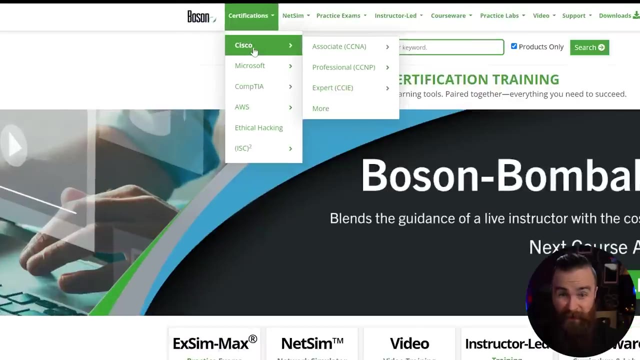 you want to get your CCNA or your CCNP- two of the best IT certifications in the world- Boson is what you want to use: From courseware to labs, to practice exams. they have you covered. They'll get you prepped and ready. I personally used Boson to pass my T-shirt exam, which is a 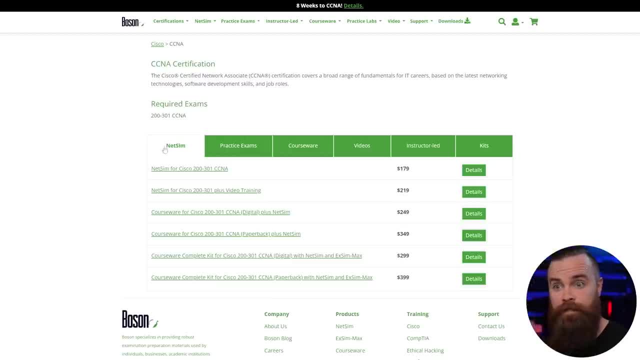 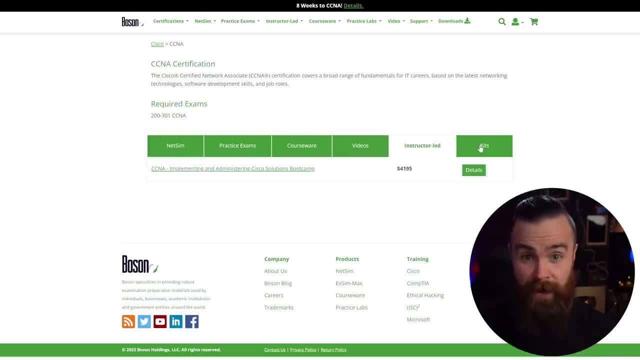 very, very hard Cisco networking exam And Boson was amazing. And not to mention they have a great amount of content on subnetting. So as you're watching this video and this series and you want to get extra practice, dude, check out Boson. And it's not just CCNA and CCNP, They have Security+. 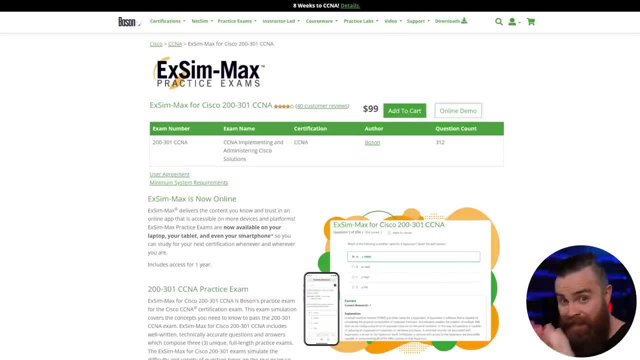 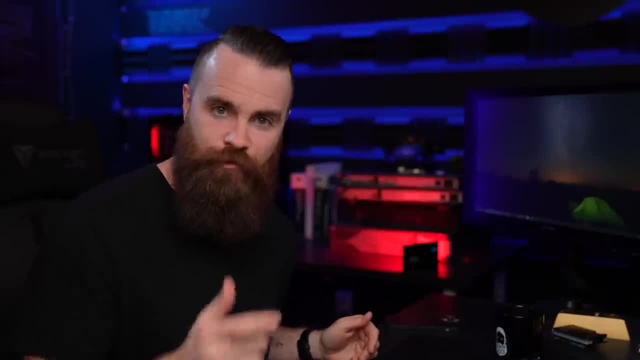 They've got CEH, all kinds of stuff. They have the best- like- I'm not kidding- the best practice exams in the industry. So if you're like, yeah, I'm not sure if I'm going to pass Security+, they'll tell you, Try their practice exam. and they'll tell you 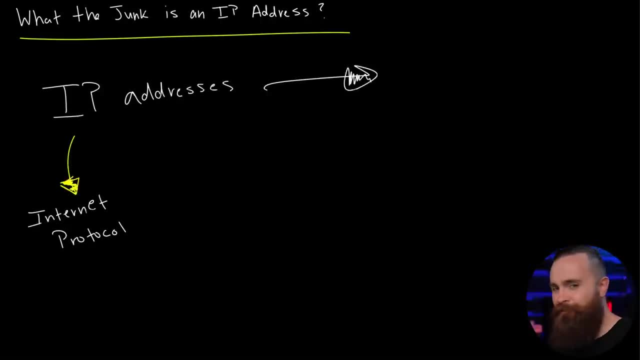 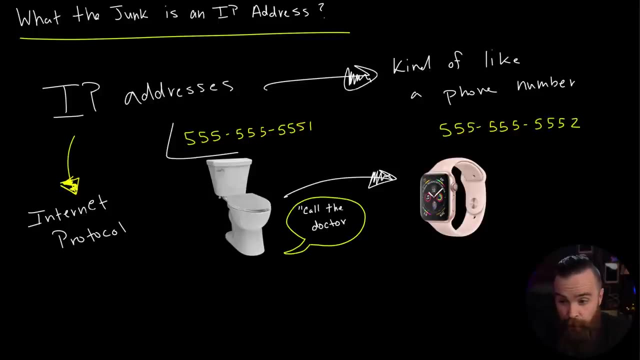 Anyways, IP or internet protocol addresses. They're kind of like phone numbers that we assign to all of our devices. So when my toilet wants to send a message to my Apple watch letting him know how I'm doing, he totally can, because they have a way to communicate with each. 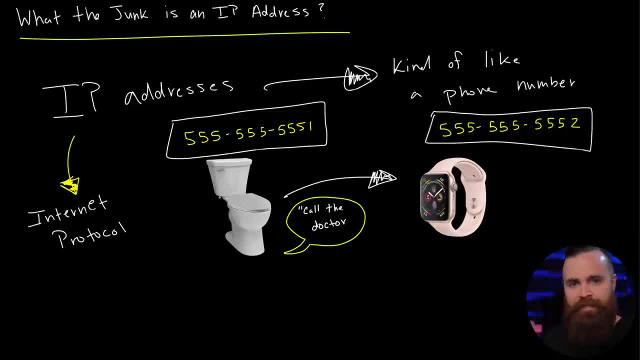 other. They have a phone number. Well, kind of We use phone numbers to text each other, but devices don't? they use IP addresses and they look a little different, for sure, And we'll talk about how weird they work, but just know that without an IP address they can't talk, So that's. 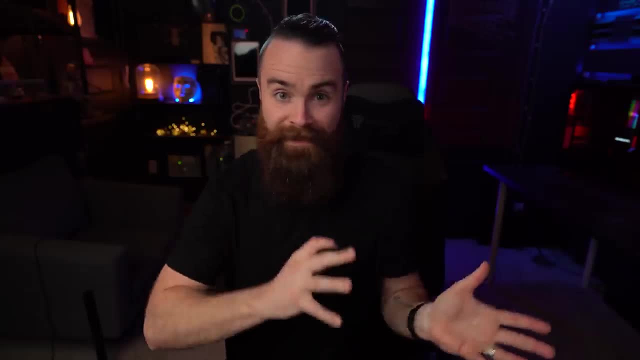 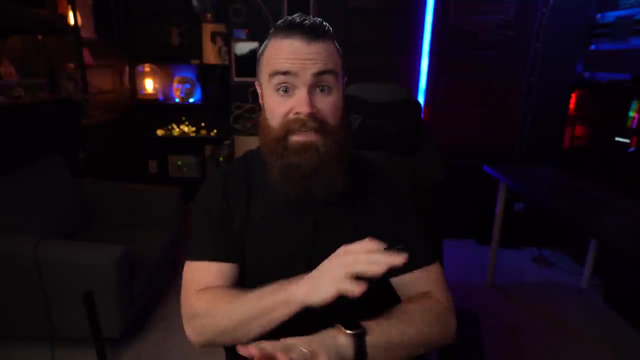 why we give them one. It opens up communication, not to mention, it gives your devices the ability to connect to the internet, because don't you want everything to be able to connect to your toilet? Yeah, So now that we know that if a device wants to talk to any other device, 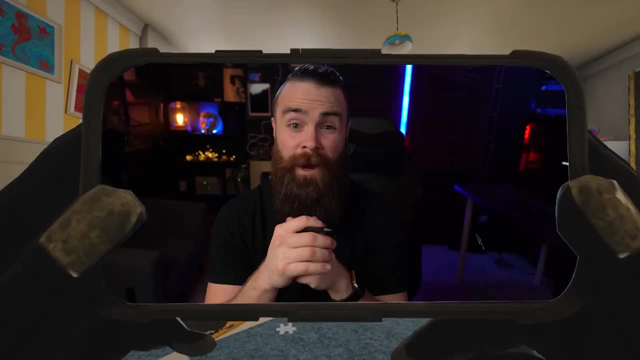 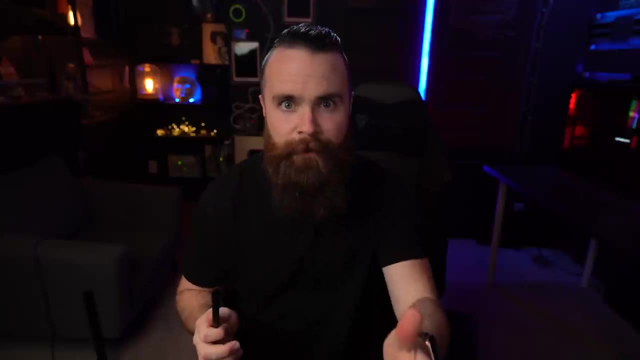 it needs an IP address. That means that the device you're watching me on right now it has an IP address because it's talking to YouTube and YouTube's talking back to it. let's go find your IP address. whatever you have, we can find it on windows. 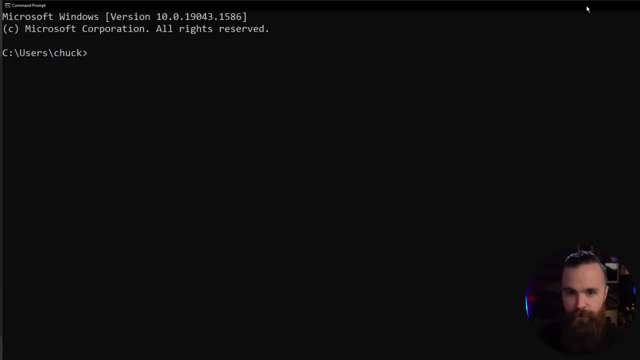 We're going to launch a thing called CMD or command prompt. go and search for that and open it. on Mac and Linux is going to be a thing called terminal. launch that And for your phone or any other device, I'll show you here in a second. here in windows, one command type in IP config. 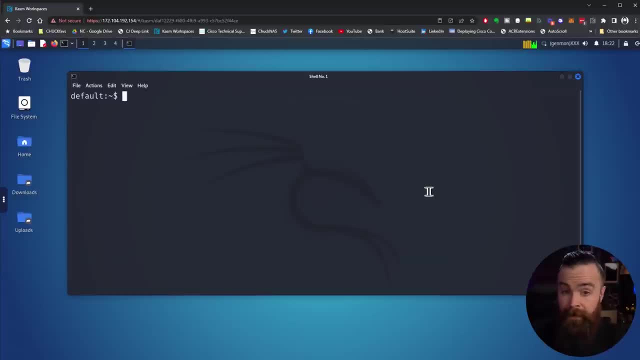 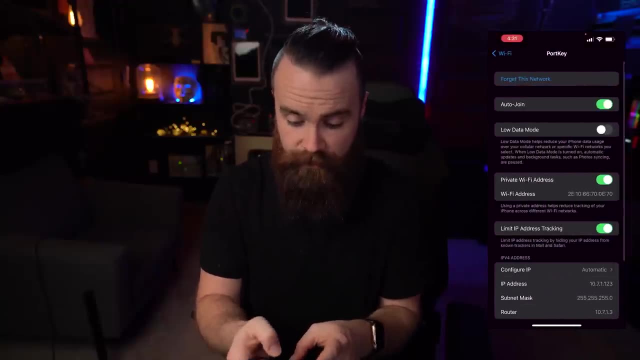 all one word, just like that, And hit enter on Mac and Linux. type in I F, config. all one word. hit enter on your phone, go into your settings, jump into your wifi info, dive deeper into that interface And you will see. Hey, there's an IP address And looking. 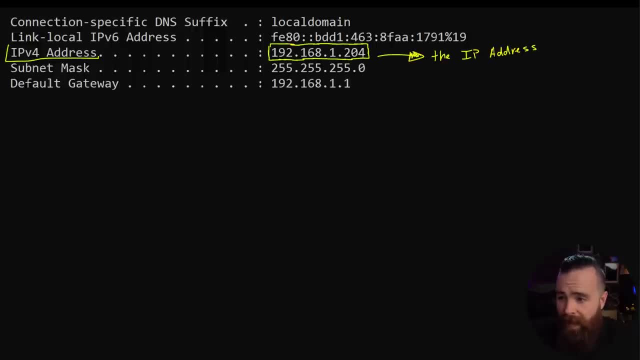 back at windows. here is the IP address. You'll know it because it'll say IPV4 address on the side over here. Don't let the V4 confuse. you ignore it for now. Now let's talk about the sucker, the IP address. He looks kind of weird, kind of dorky technical. He's a mess of numbers separated. 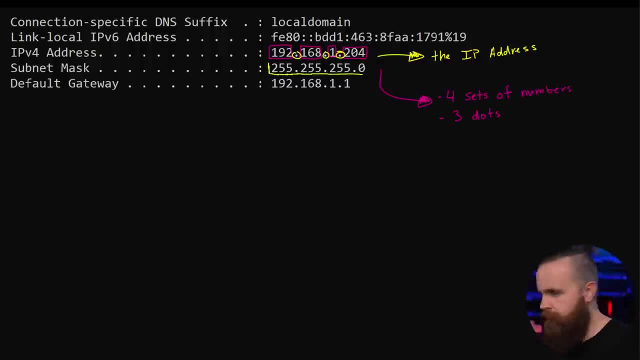 by dots, three dots. So that's already strange by itself. but then we have this guy And then this guy. what are they doing? Well, they are basically your IP addresses, best friends. We'll talk more about them here in a bit. but this guy right here is Mr Subnet mask, At least 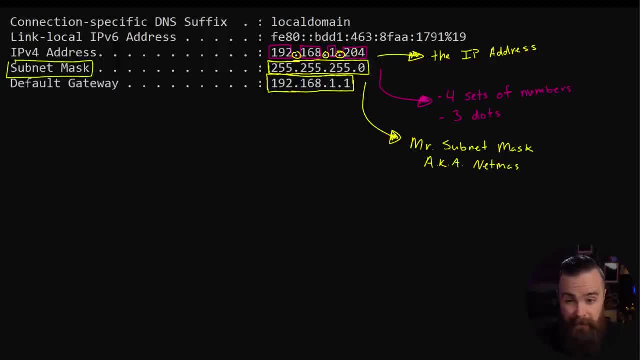 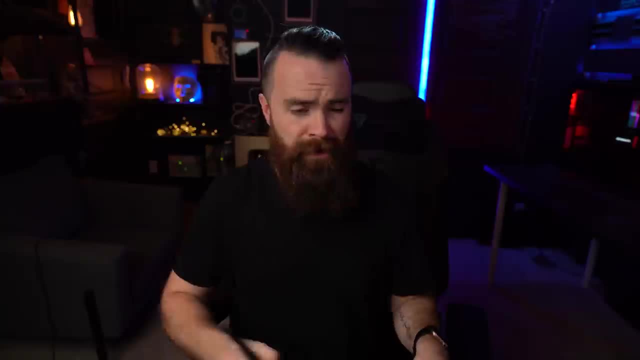 that's what he's called in windows. over here on Mac or Linux, You might see the net mask- same thing. And then this gal right here is Ms Default gateway. She also goes by default router, or just router for short. but enough about them, Let's talk about the star. 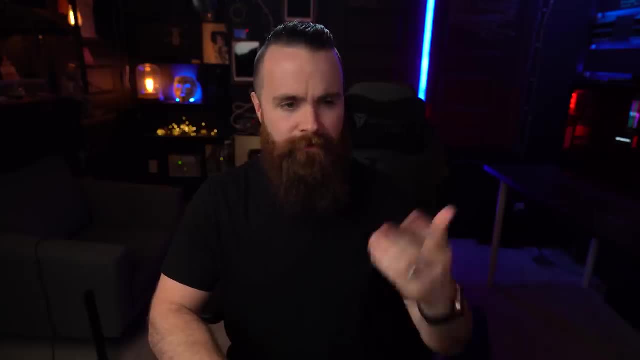 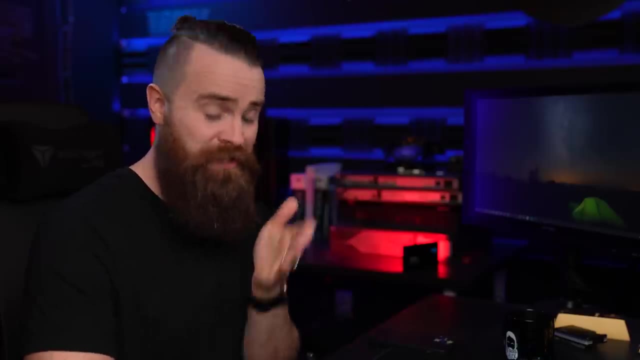 of the show, The one. we care about the IP address, And let's first cover. how in the world did he even get here? How did your device get this number? Who gave it to him? Is it safe? Who gave this to you device? Actually, that's a legit question. Sometimes you can get a bad IP address. 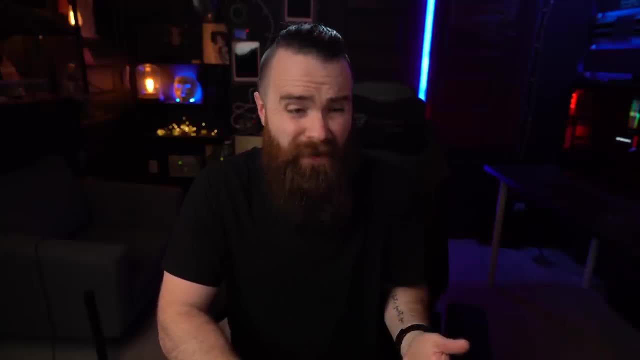 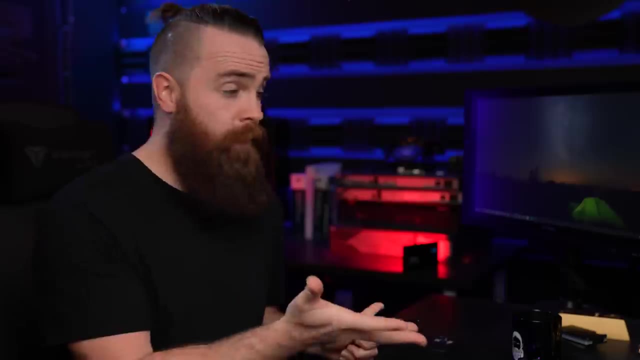 different video for another time. So how did your device get this IP address to just fall out of the sky? Yeah, kind of. If you're using wifi, you see, in your homes, in your businesses, we have this thing called a router. It may look familiar. 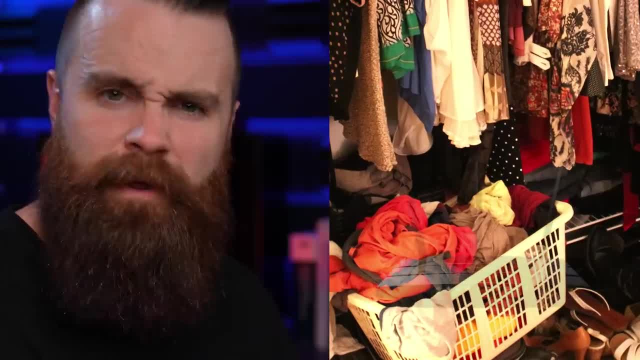 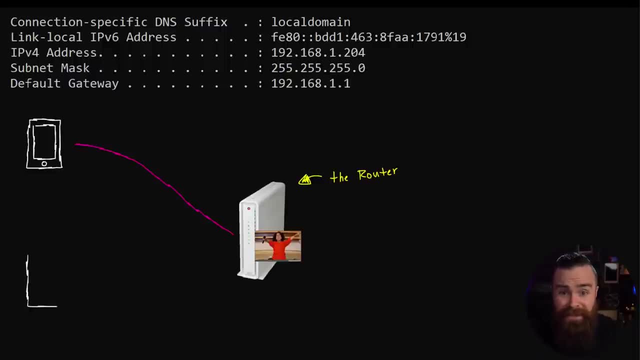 It might be hiding in your closet underneath that sweater you got for Christmas, which, by the way, rescue it. get that sweater off of him. He has to breathe. It gets hot in there. The router is the Oprah of your IP addresses. What every time a device connects to your network? 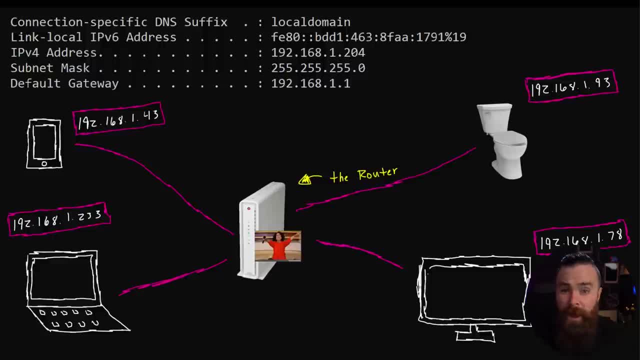 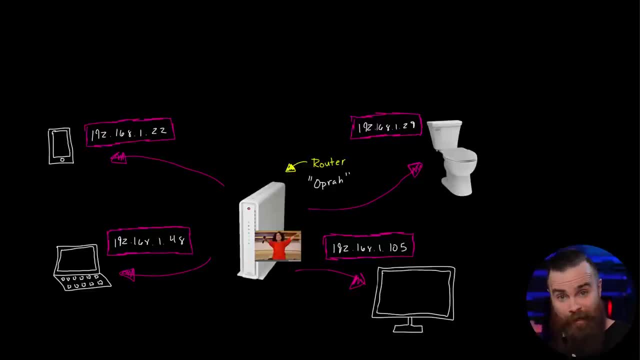 she says: here, here's an IP address, Here's an IP just for you and for you and for you. everyone gets an IP address. Now, this dark and mysterious magic known as DHCP is why this works. If you want to learn more about that, we'll talk about that later. 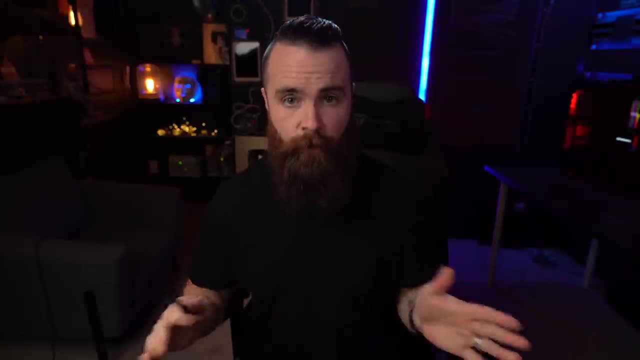 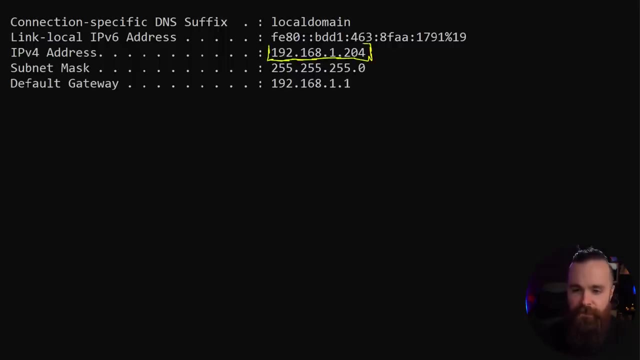 but essentially, Oprah gives your devices IP addresses. That's what I want your takeaway to be. Write that down. Okay, Now, looking back at the IP address, let me ask you a question. How is it that I know that your IP address starts with 1, 9, 2.1, 6, 8.1.. Like most of you, 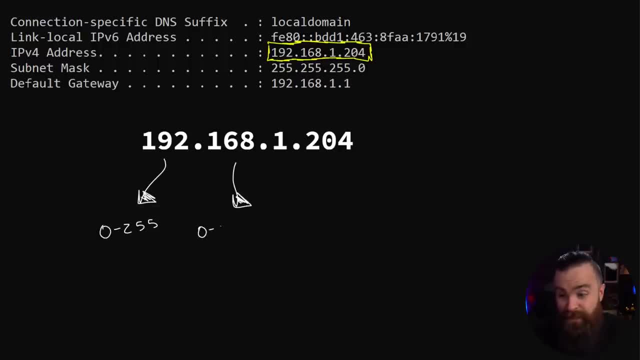 that is your IP address, right, Creepy? especially since each of these numbers can be any number between zero and 255.. So your IP address could be 10.3.2.1, or it could even be 1.2.3.4.. So why is? 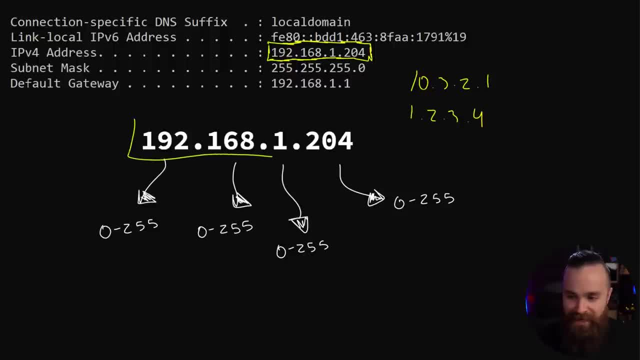 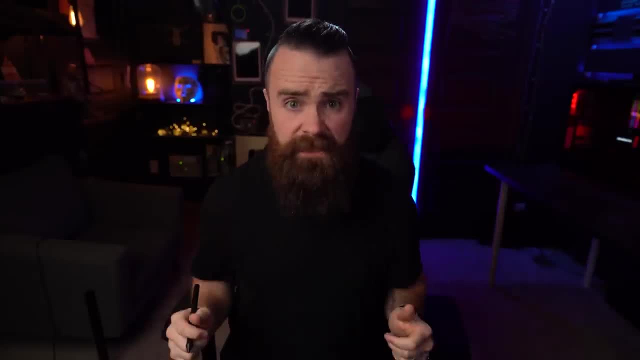 it that most of your IP addresses start with 1, 9, 2.1, 6, 8.1?? Well, there's a lot of reasons actually that I'm not gonna go into because it does get pretty complicated, but the short and easy answer. 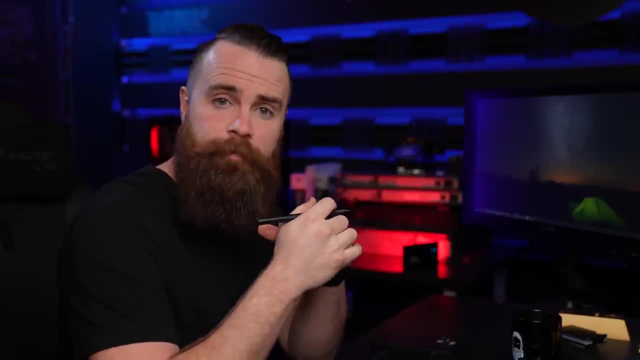 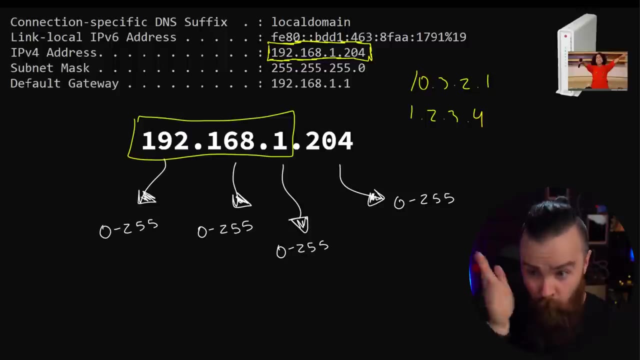 is that it's Oprah. Oprah decided that that's what your IP address should be, Should start with. It always comes back to Oprah And the way that Oprah tells us that each IP address in your network, in your house, is gonna start with 1, 9, 2.1, 6, 8.1.. It's through Mr Subnet mask, I told you. 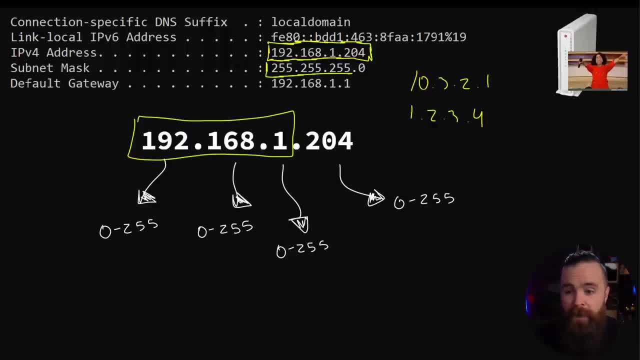 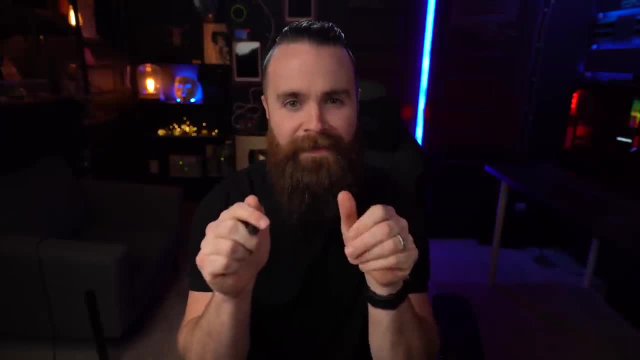 you come into play here in a bit. Here he is. He looks even weirder than the IP address And honestly he's a pretty complex dude. We're gonna spend a lot of time getting to know this guy in this series, but, real quick, can I show you a hack That's gonna save you like? 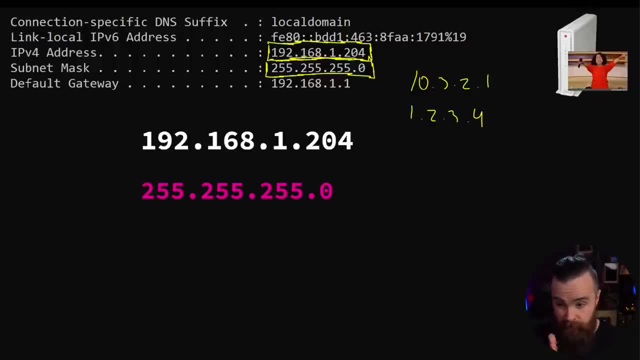 a billion hours. Now notice that Mr Subnet mask does look pretty similar to the IP address. He's got four sets of numbers and three dots, And if you assume that the first number in the IP address matches up to the first number in the subnet mask, you'd be exactly right. 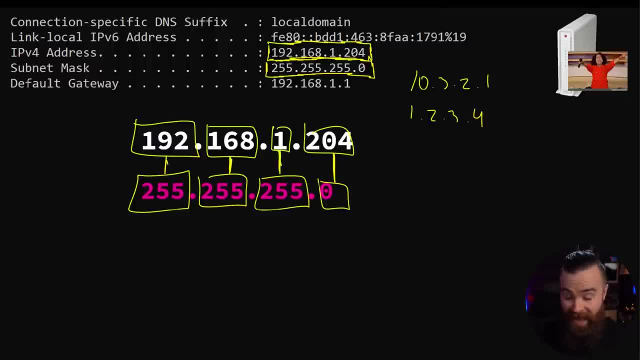 In fact, they all match up: two to two, three to three, four to four. Now here comes the hack, When you see a 2: 55 in an octet which, by the way, each of these sections separated by a dot. 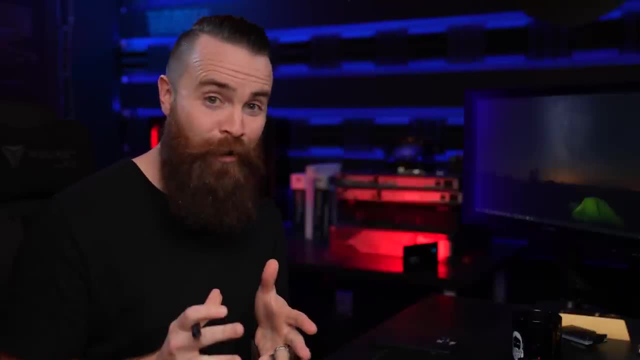 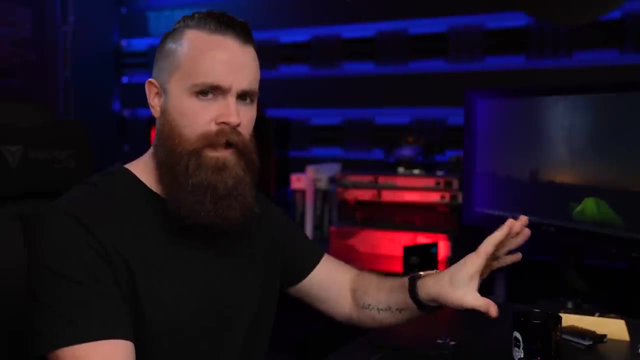 we call them octets. We will dive deeper into why we call them that. And yeah it's, it's gonna get more nerdy and so much more fun. I can't tell you more. Just know they're called octets for an. 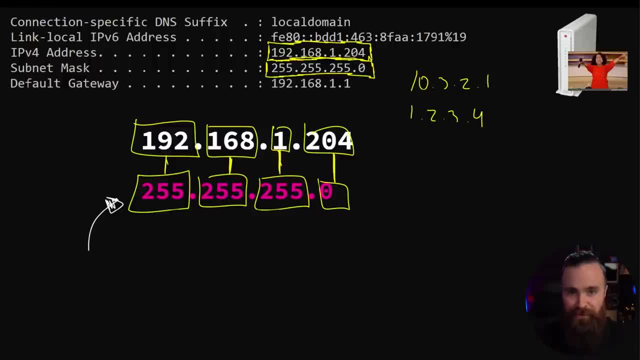 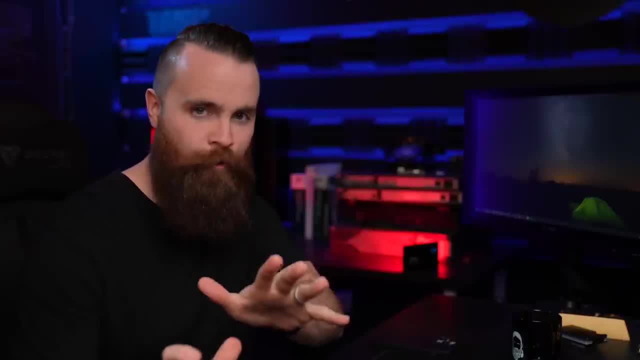 ounce Calm down. So anyways, back to the hack. If that number is a 2- 55, then we know that the corresponding number or the corresponding octet will always stay the same within your network. That is So looking at our subnet mask. here we know the first three octets, or the first three. 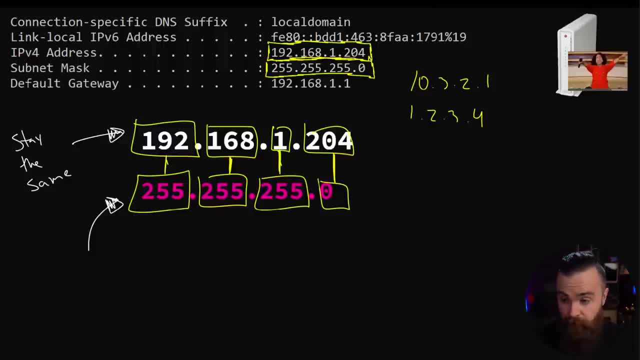 numbers are 2- 55,, which tells us that the first three numbers in our IP address- 1, 9, 2, 1, 6, 8, and one- will always stay the same in our network. We can confidently say that every single device in your network, at your house or your business, if they look like this: 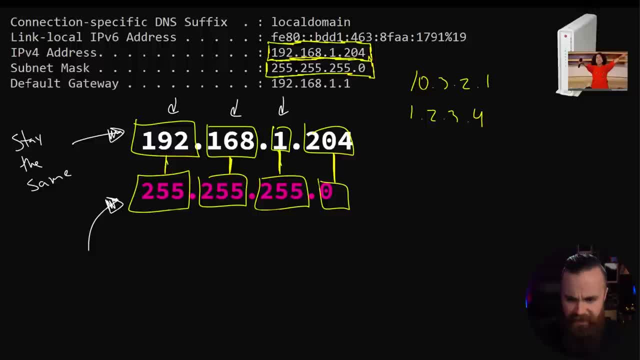 they're gonna start with 1, 9, 2, 1, 6, 8, 1.. And that brings us to the last number over here, the zero. What's this guy doing? This zero is telling us that. Hey, this last number. 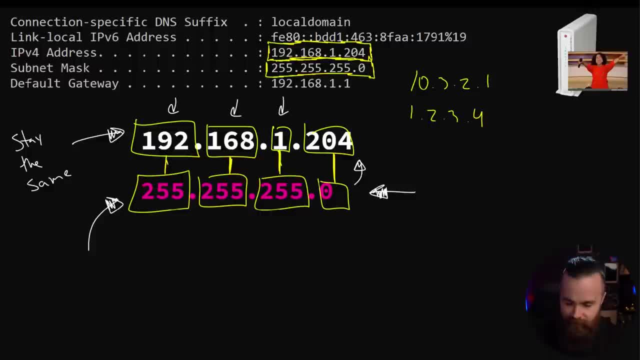 it can be whatever you want, whatever your heart's desire, as long as it's between zero and 2- 55, but still, whatever you want, you can use them all. So, to sum it up, when you see a 2- 55,, 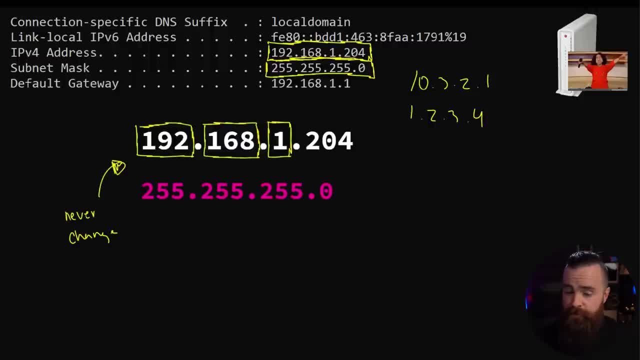 that number's locked in. These numbers will never change, but the zero tells us the final number totally will, based on what device it's assigned to. So if you allow me to get a bit nerdier and go a bit deeper in the networking world, we refer to these numbers right here as the network portion of. 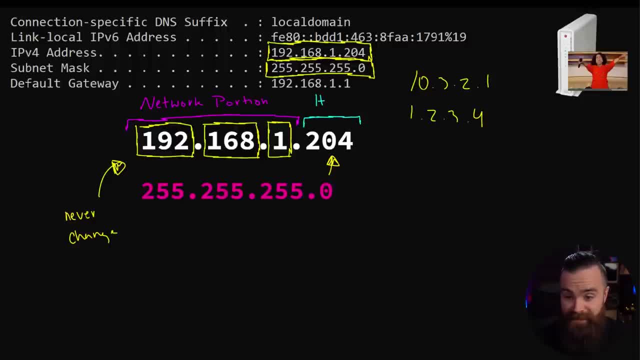 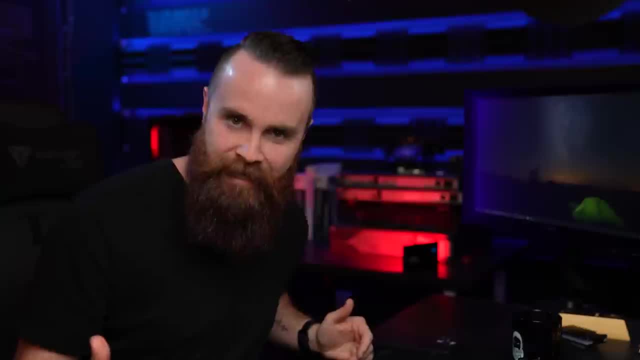 the IP address And then on this side, the side that'll change based on what device it's assigned to. We call that the host portion, because in networking and it in general, when we have devices on a network- your phone, your watch, your toilet- we call those hosts Your toilet. 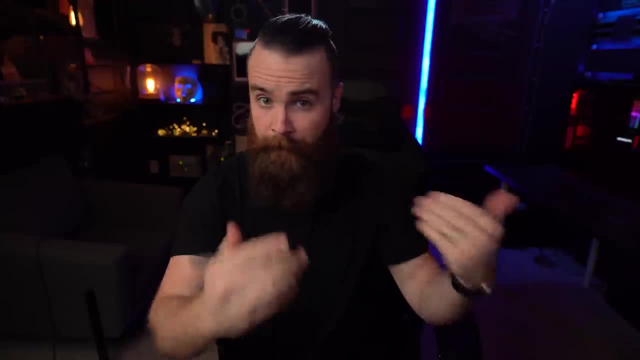 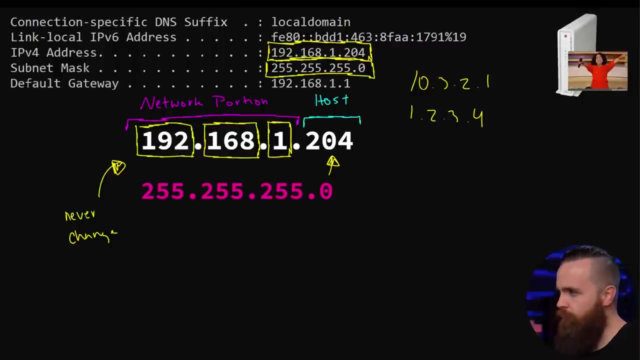 is a host and it has an IP address. Now, what I just explained: put that in your pocket. Don't let nobody hock it. This will become very, very important later. But now let me ask you a question. Why is it important that we have to know the network portion of the IP address? Why do we? 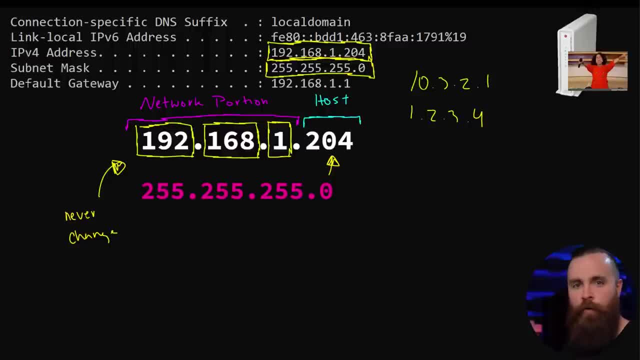 have to know that the IP addresses in our network start with 1, 9, 2.1, 6, 8.1 analogy time. We can also think about an IP address like the address of our house, like you know, the place you live. 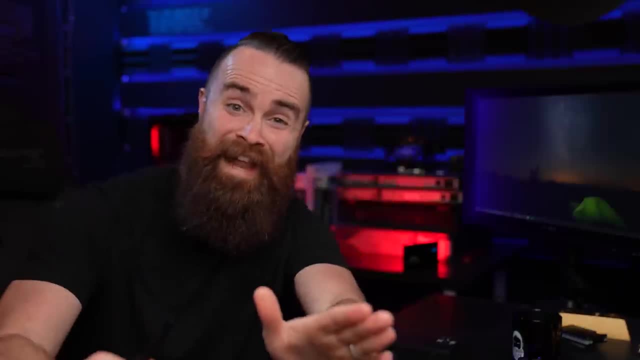 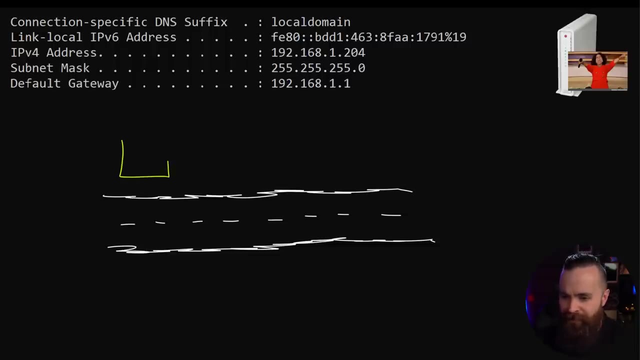 and tell you what. why don't you comment below your home address? No, I'm totally kidding, Don't do that. Are you crazy? Don't do that. But anyways, you live in a house and that house most of the time, I think always- is going to be on a street right And let's say your street, that you. live on is privet drive. If you know where that's going to be, it's going to be on a street right. If you know where that's going to be, it's going to be on a street right And let's say your street that. 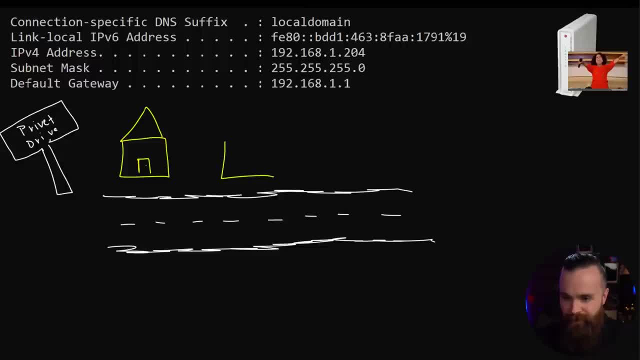 you know where that's from comment below. And because you're probably not the only house on privet drive, you can't just say, Hey, send me a package on privet drive. I live on privet drive. Oh, houses need windows. I knew it looked kind of weird, Hold on, Let me draw some windows. So 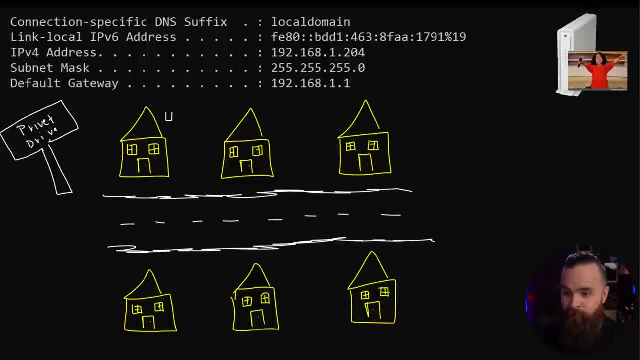 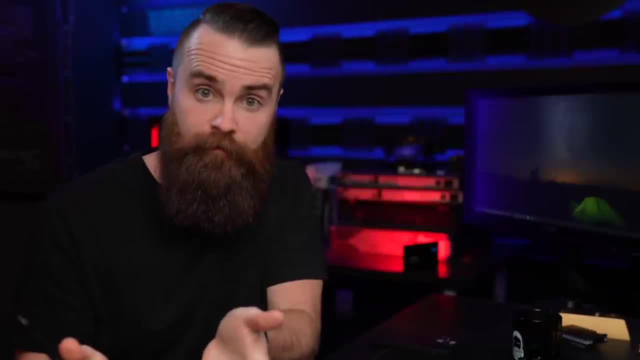 anyways, we'll assign a unique house number to you, So you might live at four privet drive and your buddy might live five and then six, then seven, eight, nine. You got it right. So if I were to send you some network Chuck coffee it would go to four privet drive. So I sent you some. 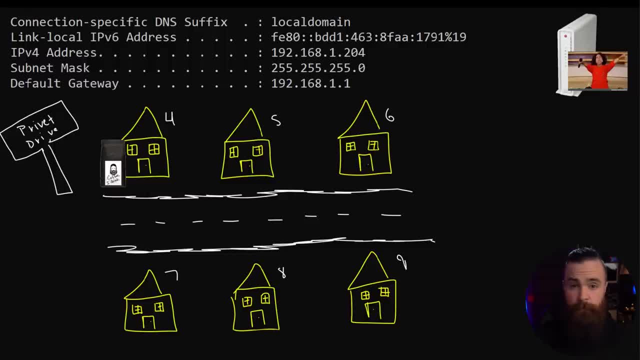 coffee and it was so stinking, dang delicious that you wanted to bring some over to your friend, your buddy Bernard, over at six privet drive. There's Bernard. Now hang tight. Here's where the analogy comes into play with IP addresses. So would you call UPS and say: Hey, I have some coffee, I want. 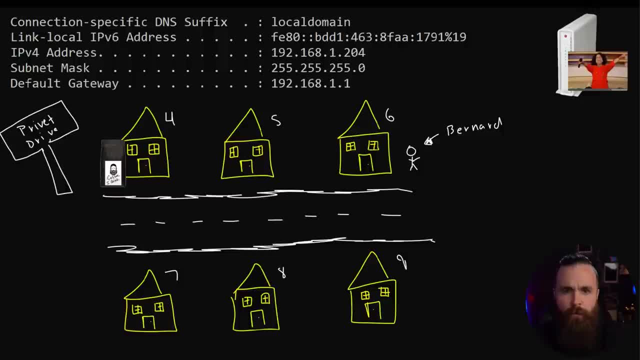 to give Bernard. come pick it up and take it to Bernard. No, no, Why would you do that? Bernard lives on your same street, So as you're preparing to send Bernard some coffee, you go. Hey, Bernard lives on privet drive, Therefore I can just walk outside and hand it to him because we're so. 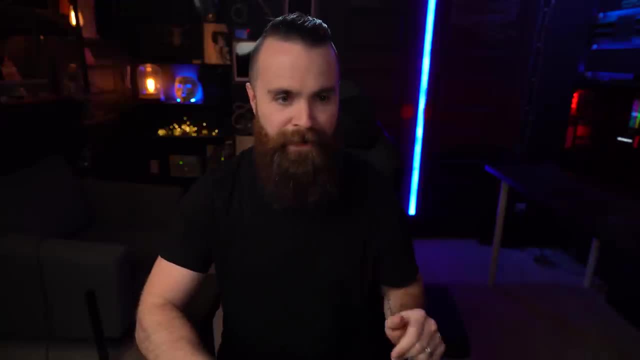 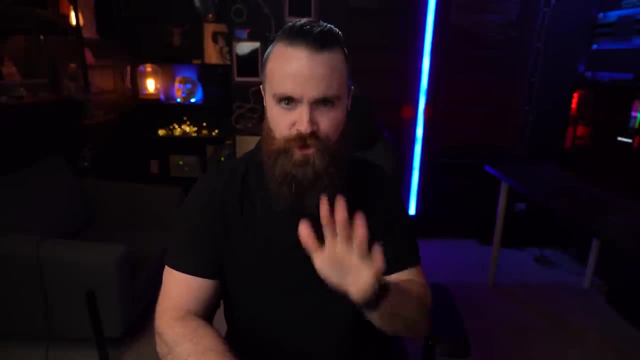 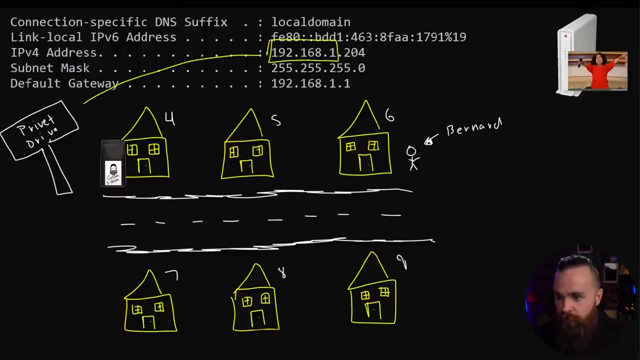 This analogy feels weird, I don't know Why. is it me? It's probably me If you're tracking with me the network portion of our IP address. the thing that stays the same is akin to privet drive, And the host portion. the thing that does change is the house address, the house number four. 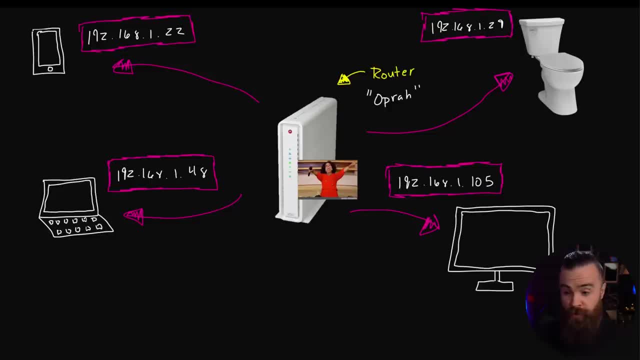 or it could be five, or it could be six, based on who you're sending it to. with our devices in our network, It's the same thing. If you want to share a picture from your phone to your computer, your phone will look at the IP address of the computer and go: Oh Hey yo, we're on the same network. 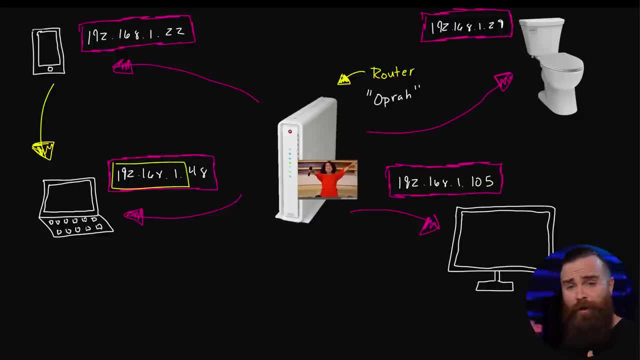 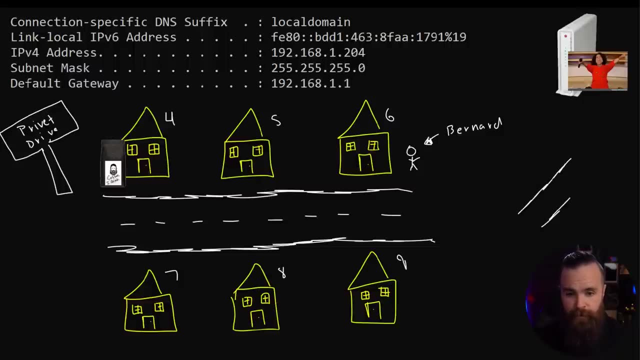 One at two, one, six, eight dot one. He's in my neighborhood, I can just walk over and give it to him. But now let's say that the coffee's really, really, really good And Bernard wants to send it to his buddy, Dr Strange, over here on bleaker street. So Bernard looks at Dr Strange's address. 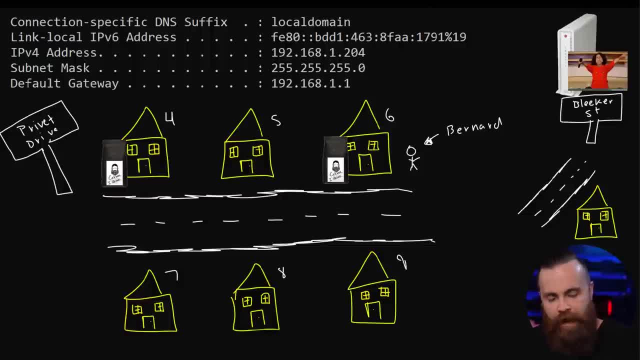 and he goes: okay, bleaker, bleaker street. I don't live on bleaker street. I can't just walk outside and hand coffee to Dr Strange. In fact, he lives all the way in New York. He's far away. 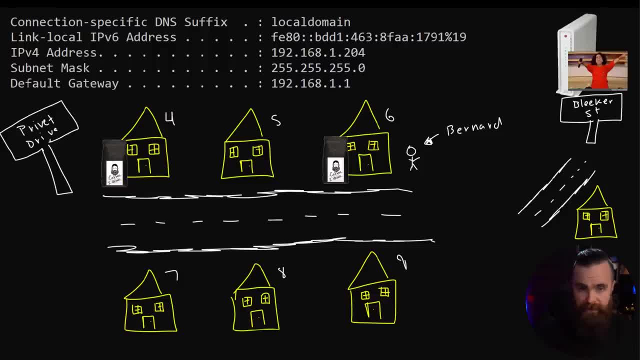 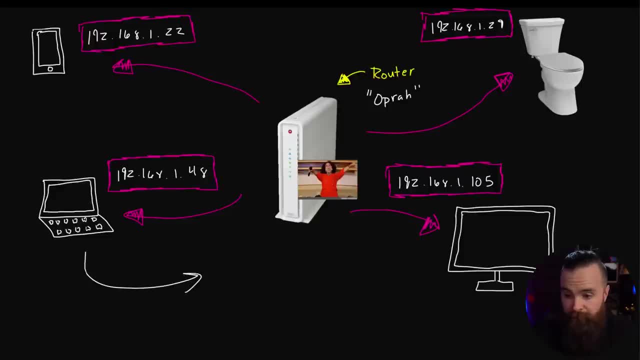 or maybe another dimension, I don't know what. what's going on? So, Bernard realizing he needs help, We'll just call UPS and have them come pick it up And take coffee to Dr Strange And, in the same way, my laptop may want to go out to netflixcom. 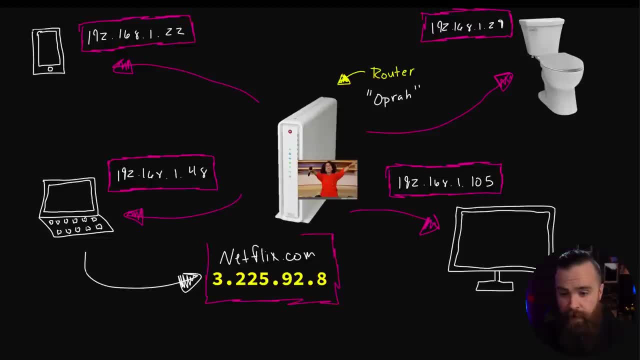 which has this IP address and it's in a completely different network And my laptop will go dude. he's not in my network, He's not my same neighborhood. I need some help. I need to call UPS, except in this scenario it's not UPS, it's miss default gateway or. 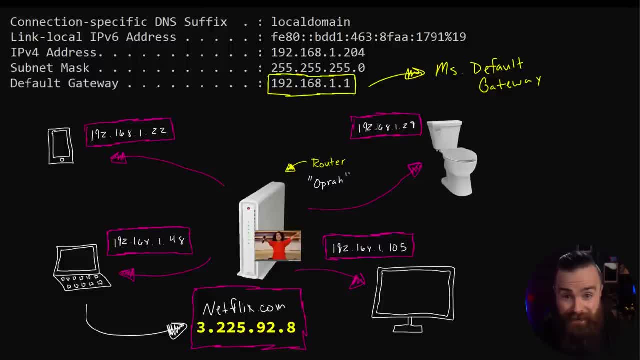 miss default router, AKA router your computer or any device on your network. We'll look at its IP address and then look at Mr Subnet mask and go huh, My network is 1, 9, 2, 1, 6, 8.1.. Netflix is not in my neighborhood. I need help. Please help me. 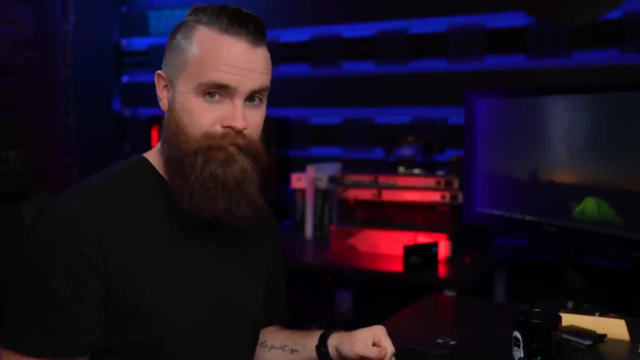 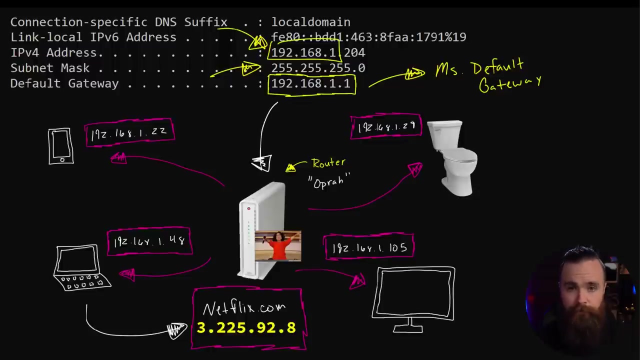 Miss default gateway. miss default gateway. She knows everything. She knows exactly how to get to Netflix and she'll take it from there. Now, fun fact, miss default gateway, She's actually your router. She's Oprah, I know, mind blown the entire time. 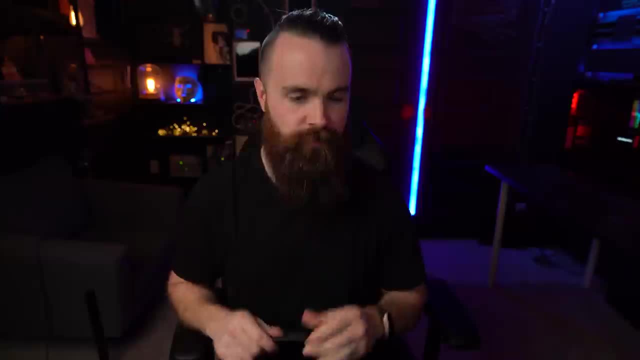 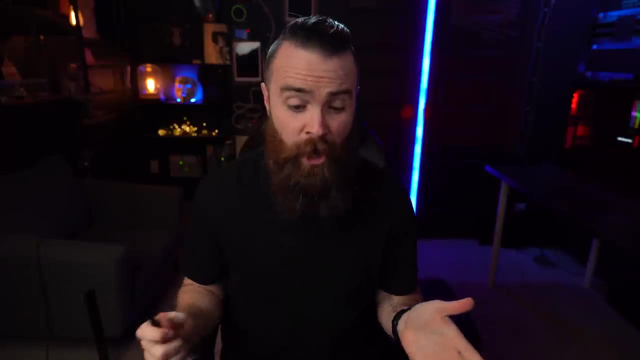 Never saw it coming. What a plot twist. That's some Scooby-Doo stuff right there. So to sum that part up, whatever any device in your network- whether it's your home network or network at a business or pretty much any network in the world- when it wants to talk to something not on it same. 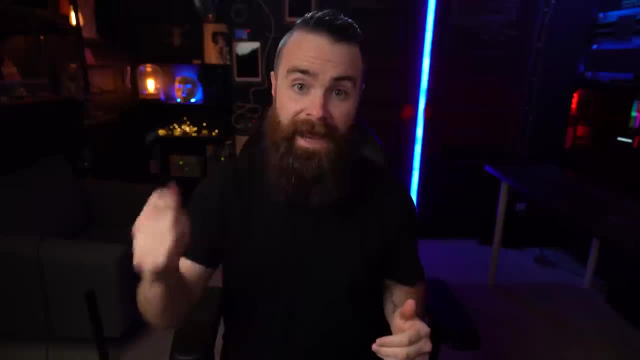 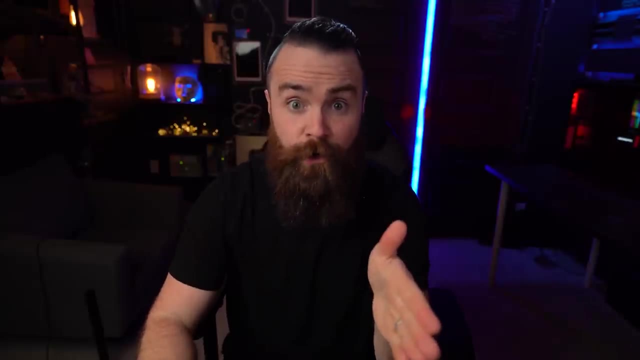 street when it wants to talk to something outside its network, it has to talk to its router, It's default gateway to get out. It has to talk to Oprah. write that down now real quick. I got a challenge question for you. Let's see if you've been paying attention. 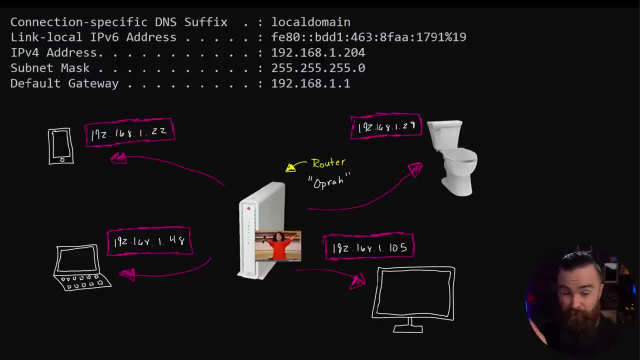 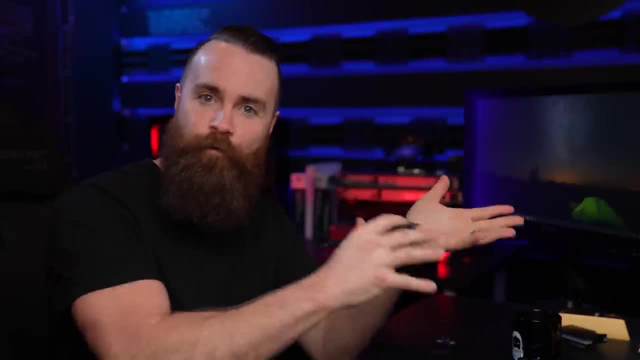 looking at my network here, which might be the exact same as your network. I told you this is one of the most common networks in the world. or did I tell you that, by the way, this is one of the most common networks in the world? My kid just screamed for private networks. Looking at this. 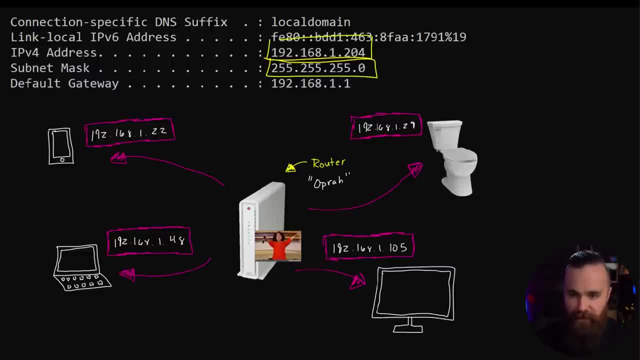 this IP address and, looking at this subnet mask, how many possible IP addresses are available to assign to devices in your network? And, by the way, if you could figure this out, that pretty much covers the majority of networks. I'm not sure what the statistics are, but I think like network. 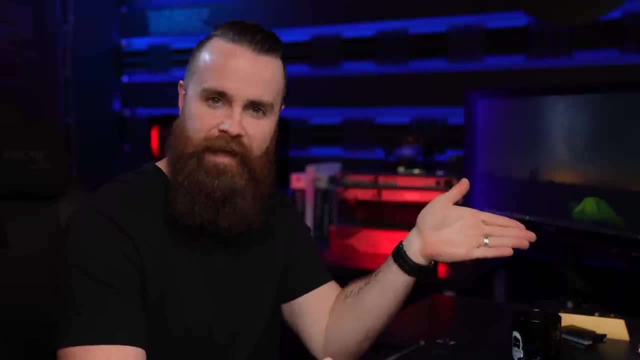 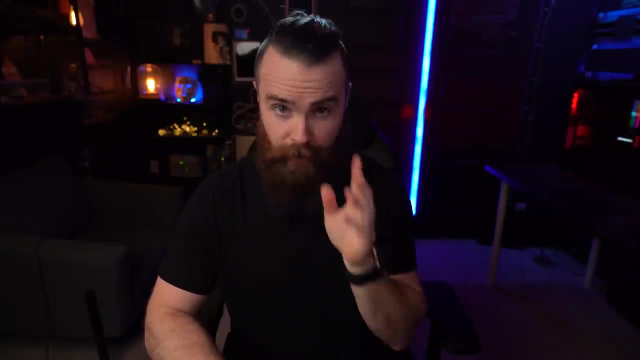 Chuck's opinion, like 95% of all networks kind of look like this. So go ahead and comment your answer below, Just raw, without me telling you. I'm curious what it will be, but let's walk through it real quick And you're probably wrong. Sorry, Looking at this. 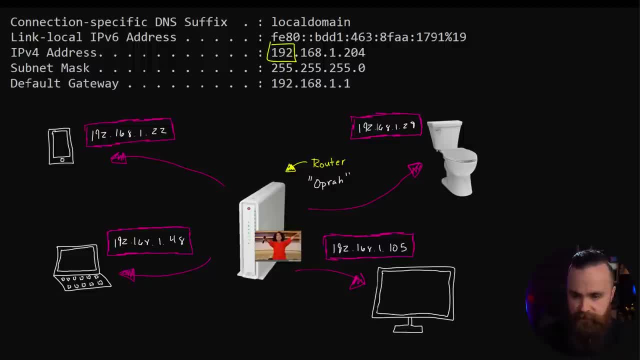 we know two five, five in the subnet mask means this number, locked in, stays the same. So does this one and this one because of the two five, five, but over here is zero. We know this last number can be anything, as long as it's between: zero and 255, which would give us a total, including zero, of 256 IP addresses party. We got a ton, but you're wrong, It's not 256, because, like everything in life, there's a catch. There's always tax, There's always extra fees. You always have to look for that. 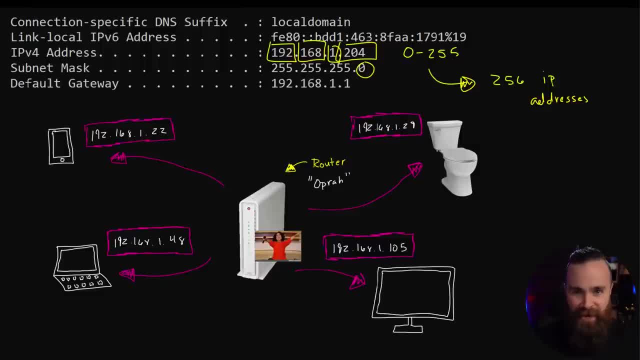 Life lesson. Anyways, here we go. Where's the catch? Where's the extra fees in our networking? Well, first of all, right off the bat, there are always two IP addresses that are reserved, that you cannot touch, You cannot use in any given network. first, 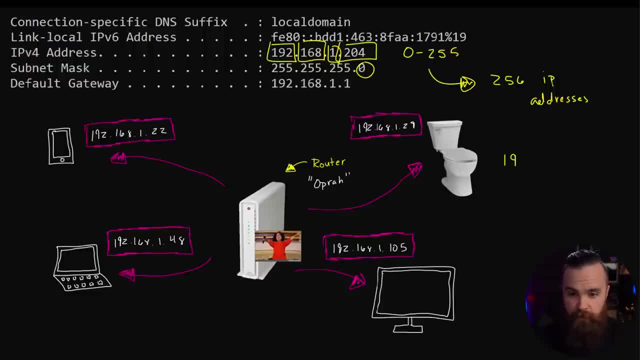 It's the first IP address in your network, So in this one it would be 1, 9, 2.1, 6, 8.1, 0.. That one's untouchable. It's referred to as the network address. He's a leader, He's the first. 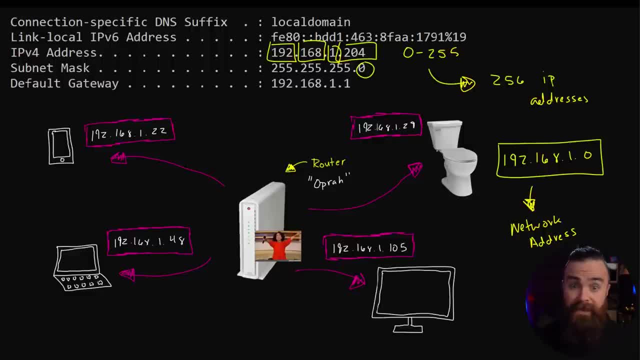 the first born son. You can't touch him. The second IP address you can't touch is the last IP address in your network. In this particular network we're talking about, it'd be 1, 9, 2.1,, 6, 8.1, dot 2, 55.. This guy, dude. 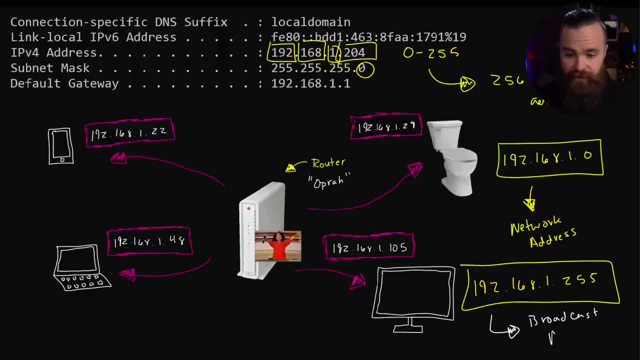 he talks way too much. He's a chatty Cathy. We call him the broadcast address because when you tell him something, he tells it to everyone, Can't keep a secret. That's legit what he does. When you send anything to a broadcast address, the last IP address. 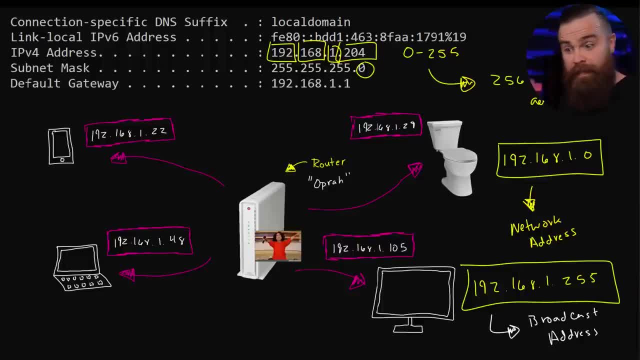 any network, it literally will broadcast it out to everybody. It's like: Hey, everyone, guess what? So don't tell him anything unless you want everyone to know. So that's two you can't touch, And then one you really have to think about and it 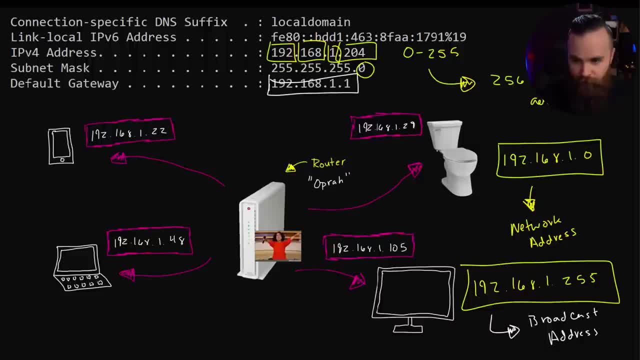 it might just be- miss default gateway. There has to be a router. Oh, I just drove over that. There has to be a router in your network and that will take up one IP address. So we're now three IP addresses shy of 256,. 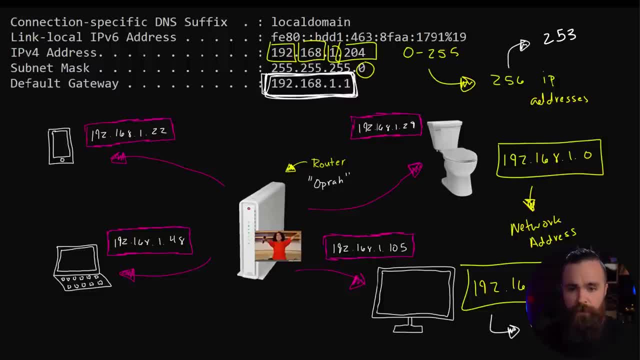 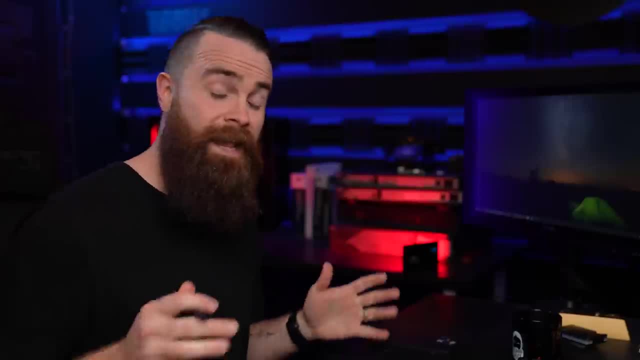 which gives us a total of 250 free usable IP addresses. If you got that right, you're on your way to becoming a sub netting master- Congrats. If you didn't, that's totally okay. This is so brand new and can be very complex, but don't worry. 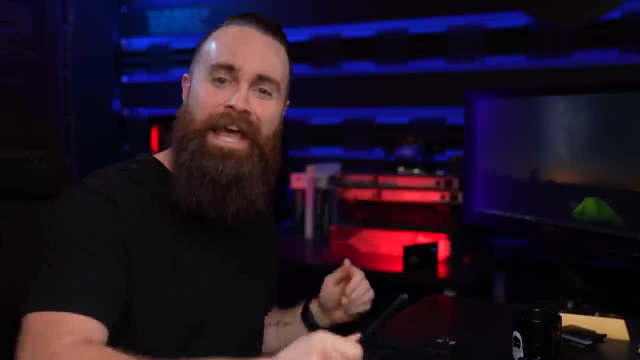 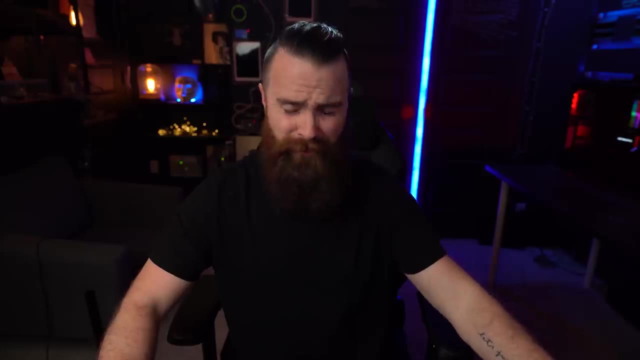 We're gonna hold hands. No, I'm gonna hold your hand. I'm gonna hold your hand and walk you through this. So little coffee break. We covered so much in this video. Oh, that's cold coffee, yet That's how long we I've been here recording. 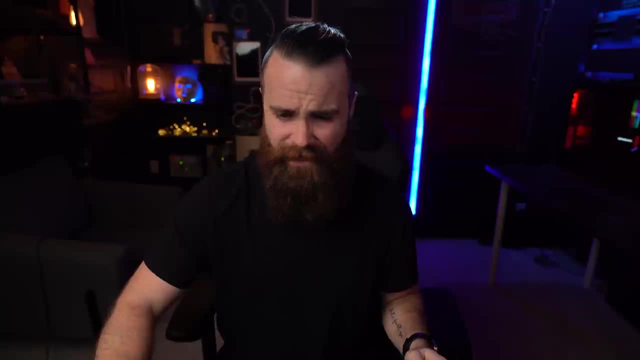 It's cold coffee, like the video, Cause I just sip some cold coffee. I I I need to go heat it up, But anyways, let's take a look at what we've covered so far in this video. We talked about IP addresses, right? 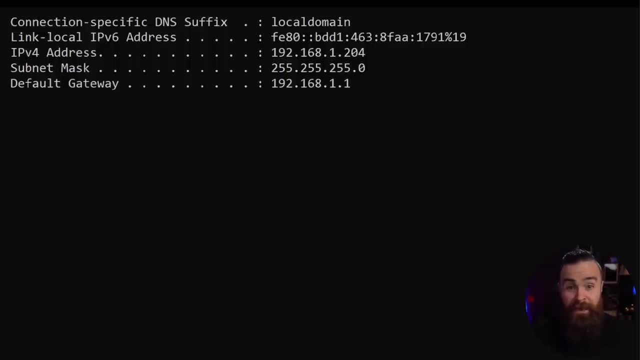 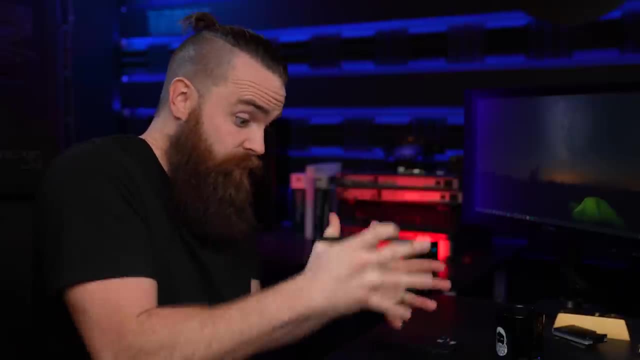 We talked about that: everything in your, your network and your house that wants to connect and talk either to other devices in your network or to devices outside the network on the internet, Netflix, or just your toilet having a conversation, a conversation with your watch. 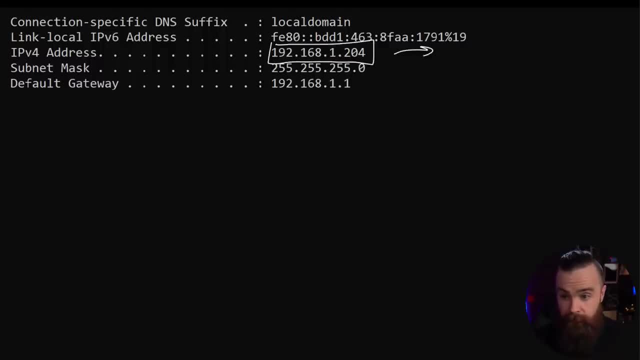 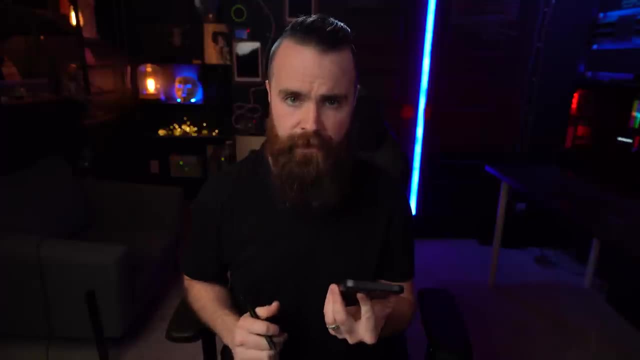 If any of that needs to happen, you have to have an IP address, basically the cell phone number of your devices. unless you actually have a cell phone, then it also has a cell phone number and an IP address. Very confusing, I know, Chuck, get better at analogies. 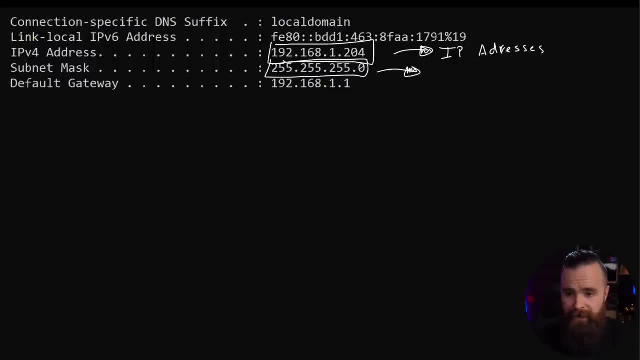 You also get a chance to meet Mr Subnet mask, a very complex and mysterious dude You'll get to know a lot better in the coming videos. He also goes by net mask and he tells us in our devices what our IP addresses in our entire network start with. 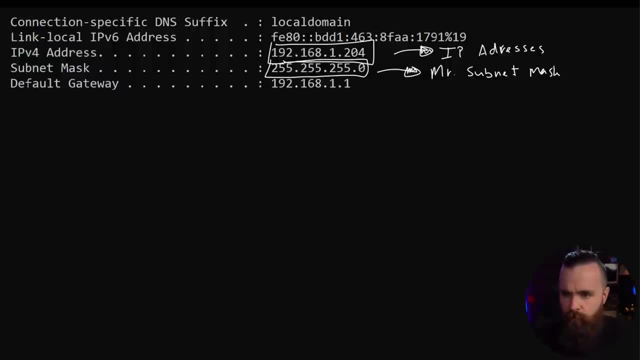 He tells us what street we live on And this network, right here, the street we live on, is 1, 9, 2, 1, 6, 8.1 because of our little hack, the two, five, fives. And then finally you met miss default gateway. 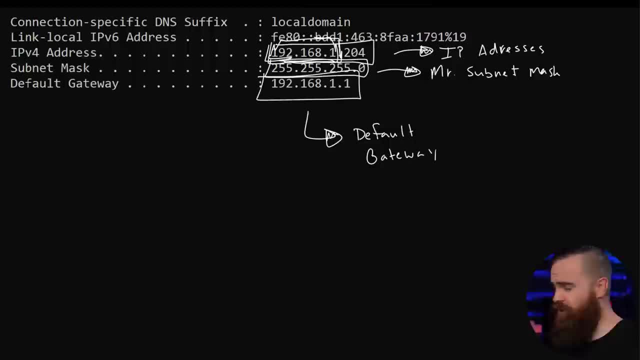 AKA default router or router or Oprah, She does it all. Not only does she give all your devices in your network and IP address, but she can help you get outside your network If you wanna go visit Netflix or network chuckcom or, even better, network. 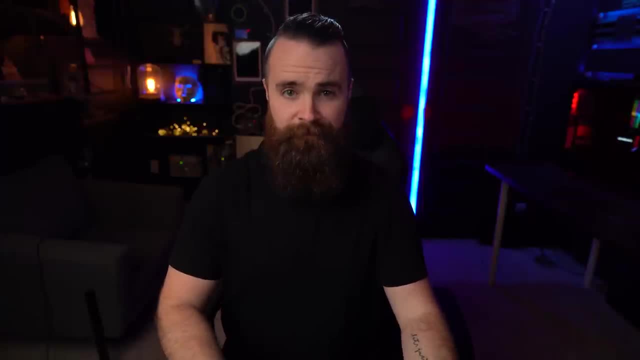 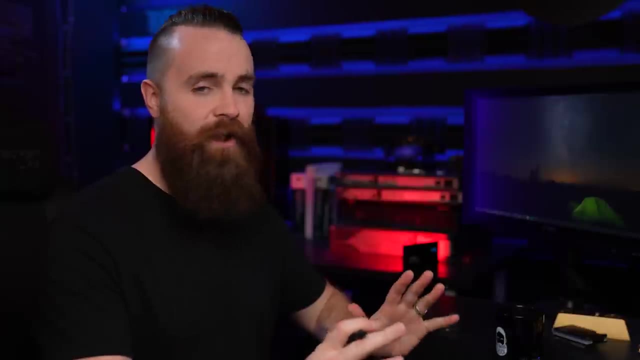 chuckcoffee. So, anyways, that's IP addresses, and I just realized I spelled IP address wrong. Let's add the extra D. cool, We're good. And let me tell you, yes, we are just scratching the surface. We're gonna get much more complex on how IP addresses work in the world. 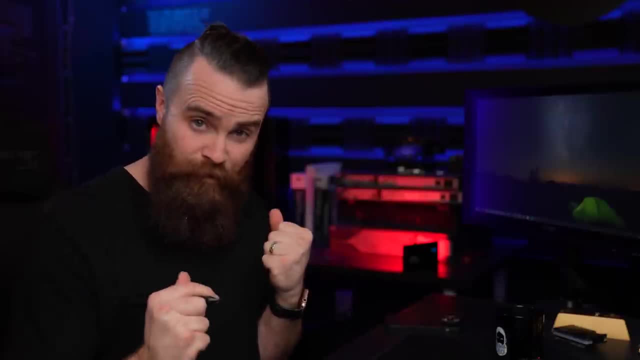 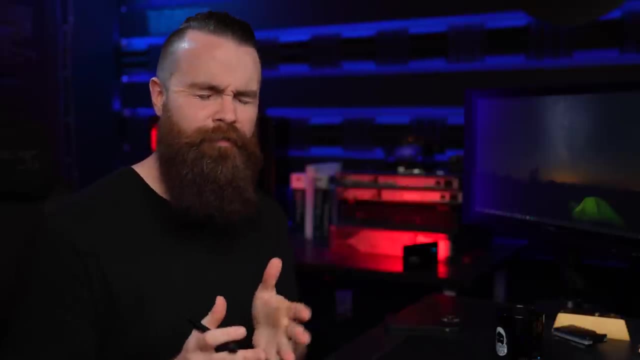 and in your home network and in your business, And you'll learn that killer skill, that crazy, awesome skill that you pretty much need for anything in it subnetting. Because let me tell you, this example we've been working with here is very, very simple, but don't you worry. 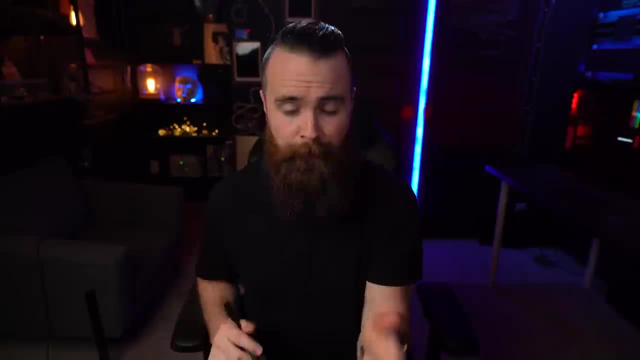 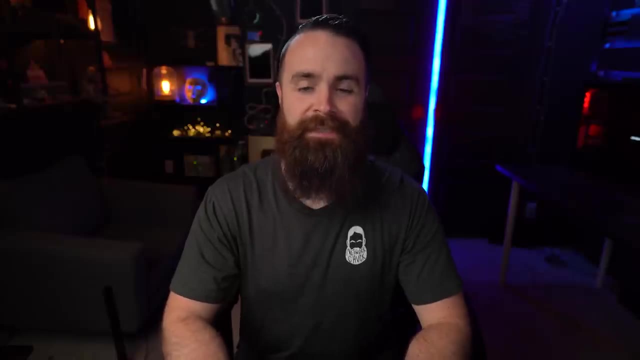 You're gonna learn the skills to make this crazy, complex and fun And by the end you will be a master, chief ninja subnetic master. Did I say master twice? That's fine. This video is sponsored by manscaped Hold on. 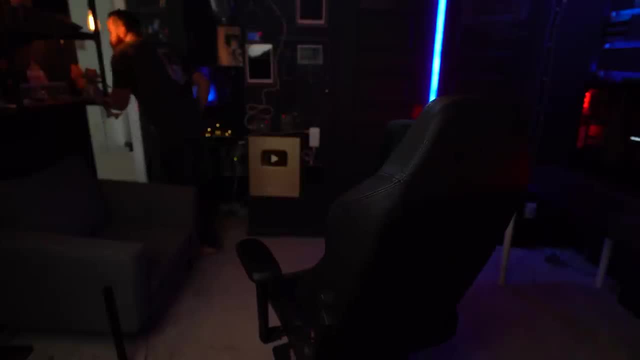 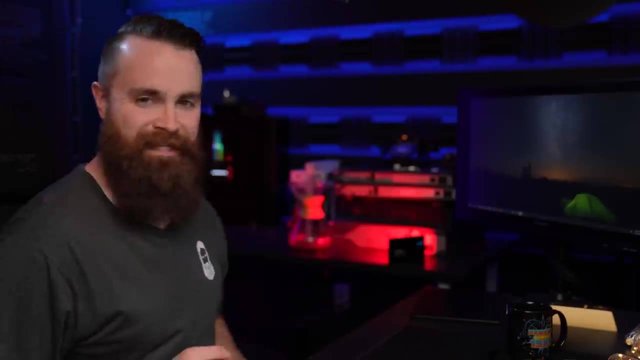 Let me just make sure there's no one listening. I'll be right quick. We should be good. No little ears out there. All right, Listen up men. This ad is for you cuz I got some new toys. So, as you may recall from my last ad or maybe other ads, 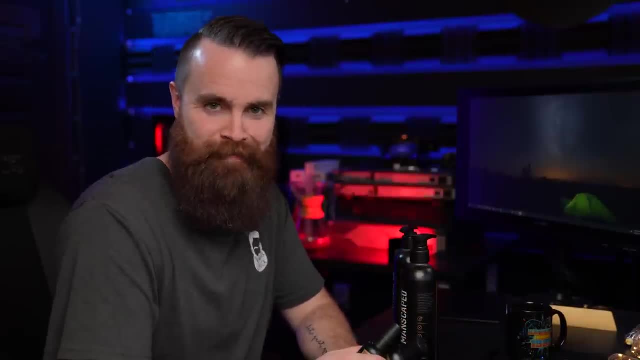 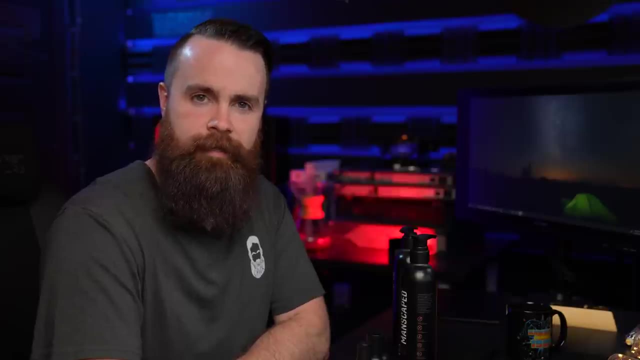 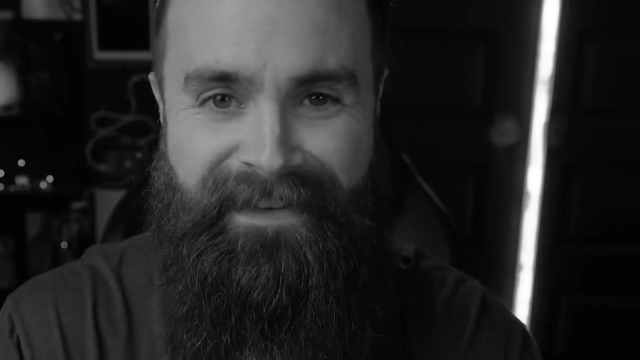 manscape is all about stuff below the waist for men. Yeah, It's trusted by over 4 million men to make sure everything downstairs is looking good, Smelling good. Now manscaped is going um beyond the groin with the brand new lineup of products. 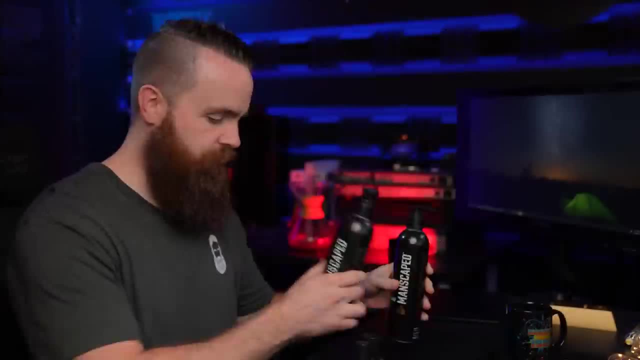 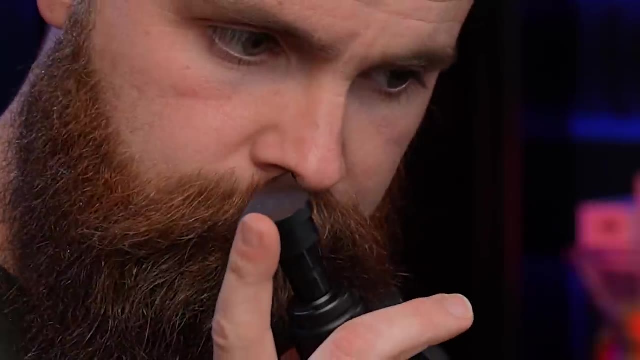 They're calling this the manscaped ultra premium collection- All those really big words. This is an all-in-one skin care kit, So they got stuff for your skin and for your hair. Smells pretty good. Got some shampoo and body wash. 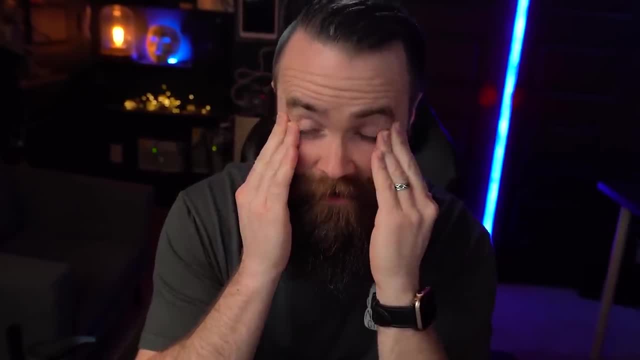 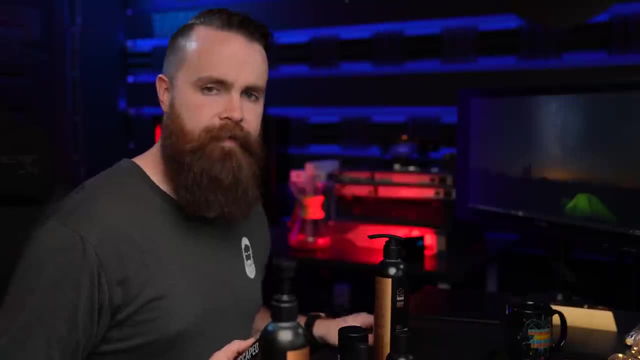 And this is the newest formulations by manscape for your- uh, your- butt, balls and body all in one package, The reason these ads are so awkward? All right, So they, they have steps. What do you say? We give it a try. 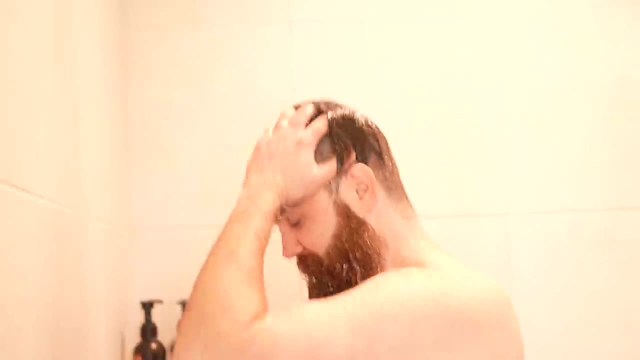 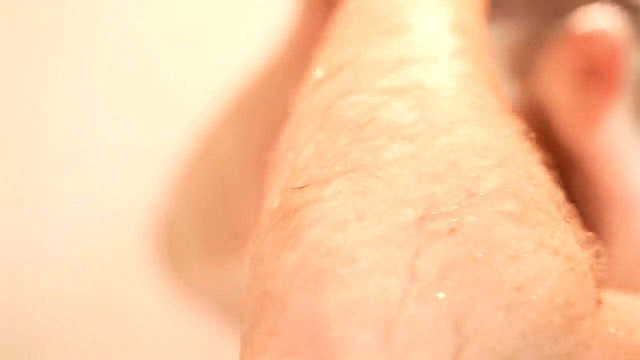 Let's do this. Step one: I'll hop in the shower and use the two in one: shampoo and conditioner which cleanses and nourishes with a luxurious lather. It's got coconut water, green tea, aloe, turmeric and sage feels nice. 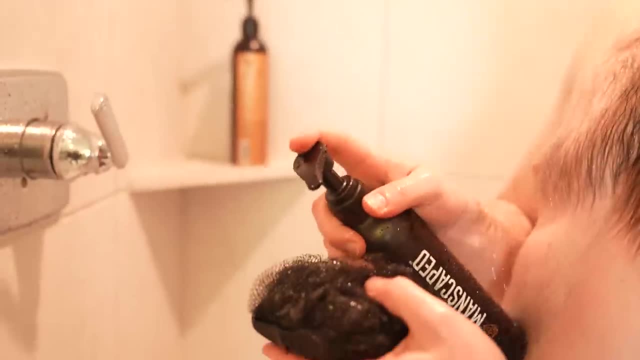 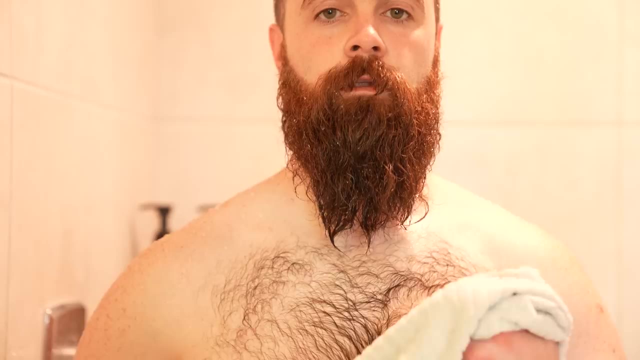 Step two: We got the body wash. The body wash is a premium daily shower gel That's infused with aloe vera and sea salt. It's the perfect balance of tough cleaning and soothing hydration. Step three: We're going to rinse and towel off and then apply something I've never seen before. 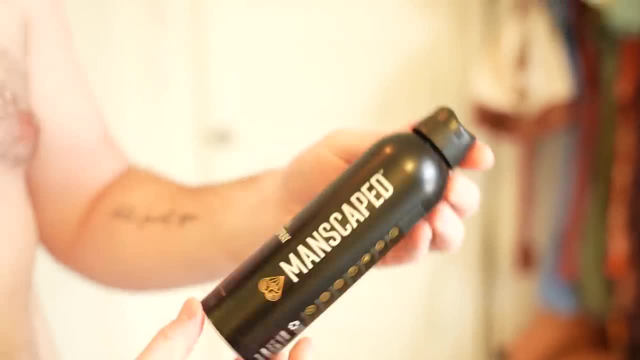 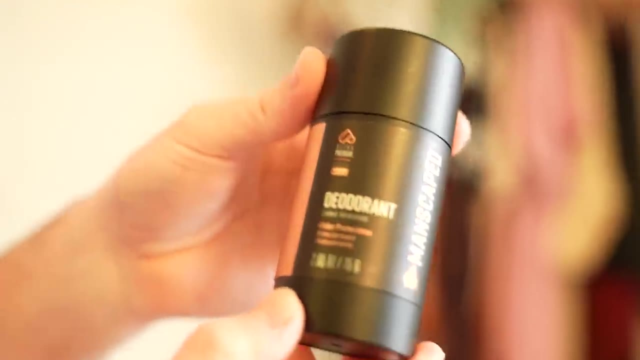 Manscaped hydrating body spray. It's a spray on moisturizer for everyday hydration. That's what it says. Got a 360 degree delivery spray system. And no, we're not done yet. Step four: We got deodorant. 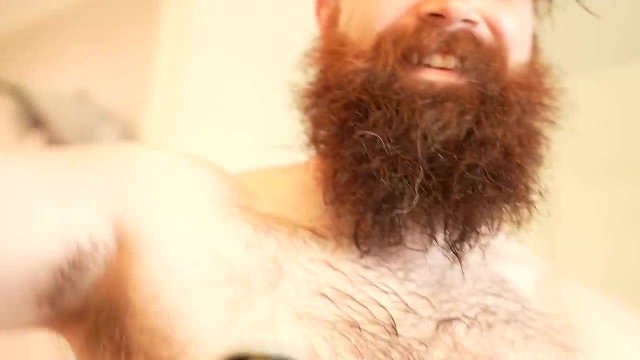 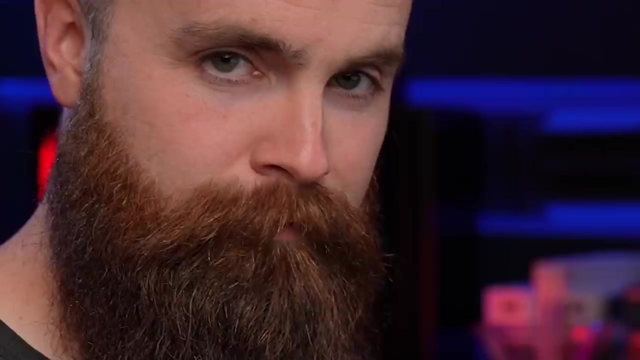 Smells pretty dang good. This stuff is stain free, Aluminum free, Drys, clear, Smells, frigging, fantastic. And now time for step five: Manscaped lip balm. You've probably never seen my lips. They're there, but my wife says I don't have any. 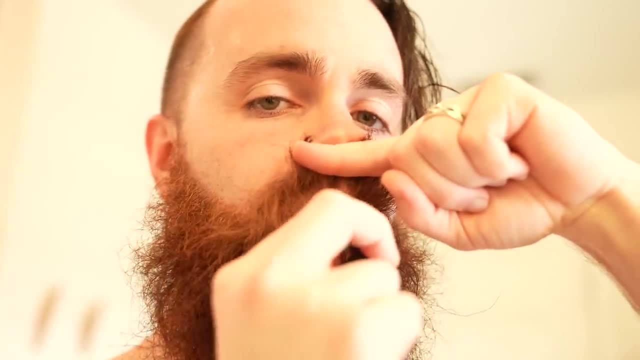 It's got vitamin E, peppermint and eucalyptus To help soothe Hypertension, Hydrate and seal in moisture. All this stuff is cruelty free, paraben free and it's vegan. And that was five steps, five minutes. 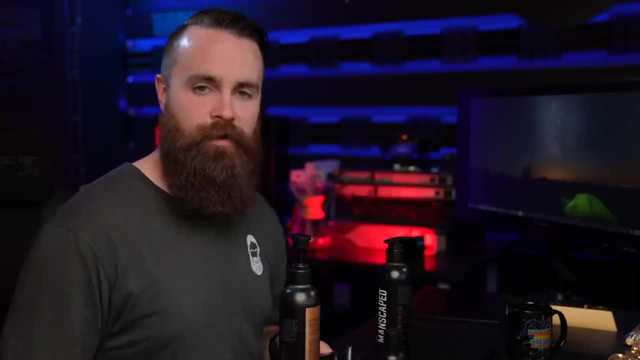 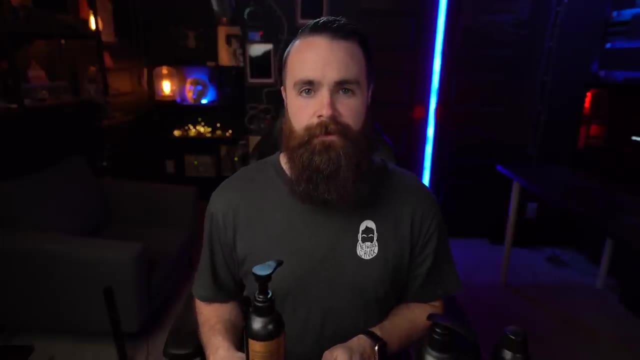 Although I like to take my showers a bit longer, So 10 minutes. Oh, you can also opt in for the Manscaped uh peak hygiene plan, So you can make sure you never run out of stuff, Cause you know I don't like going to the store. 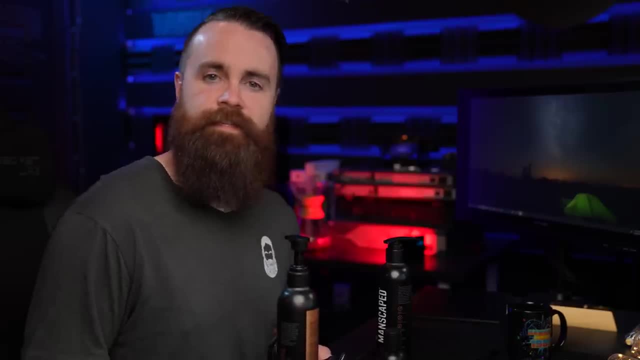 Just pick a plan and that stuff gets delivered to you without you thinking about it, So you can focus on studying and IP addressing and subnetting. Go to manscapedcom and use promo code network chuck and get 20% off your order. 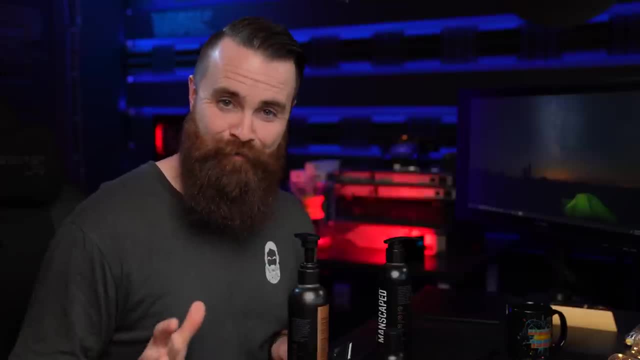 Plus, receive free international shipping- And yeah, that was 20% off with free international shipping with promo code network chuck at manscapecom or just click the link below. Thank you, Manscaped, for covering me head to toe And seriously thanks for sponsoring the video. 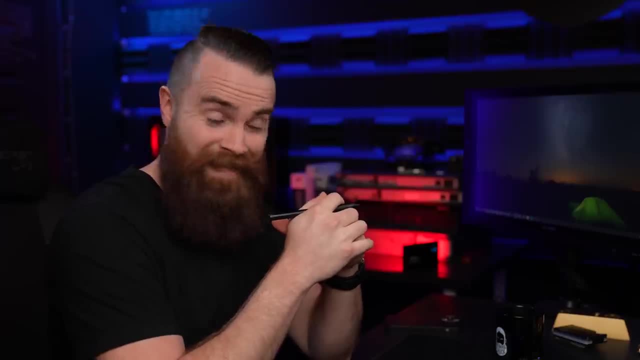 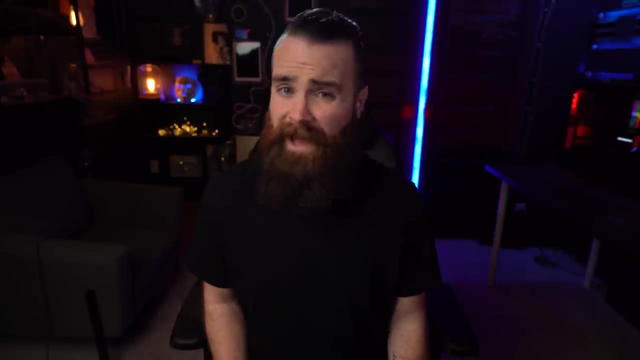 You guys should get this stuff, Cause you stink anyways. but that's all I have explaining. IP Addressing is not easy, So let's make sure you hack the YouTube algorithm today. Hit that like button. subscribe notification bell comment. We gotta hack YouTube today. 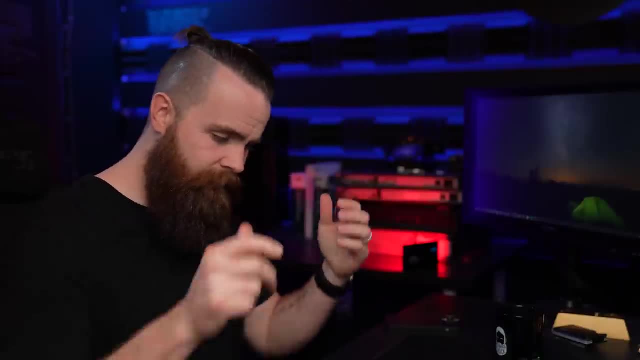 Ethically, of course, And yeah, that's really all I got. I'll catch you guys next time.